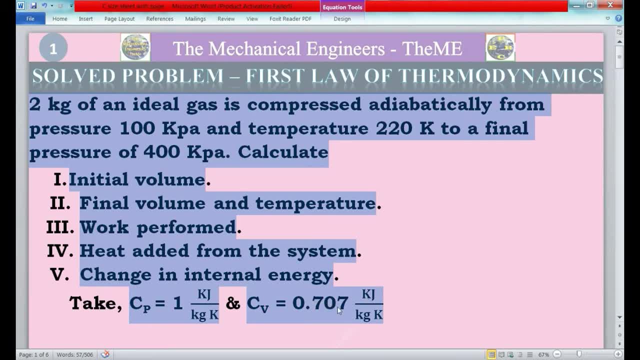 is equal to 0.707 kilo Joule per kg Kelvin. Now I will analyze this question. 2 kg of an ideal gas has been compressed and the compression of gas takes place during adiabatic process. which means In compression process heat will not be added to the gas and also heat will not be rejected. 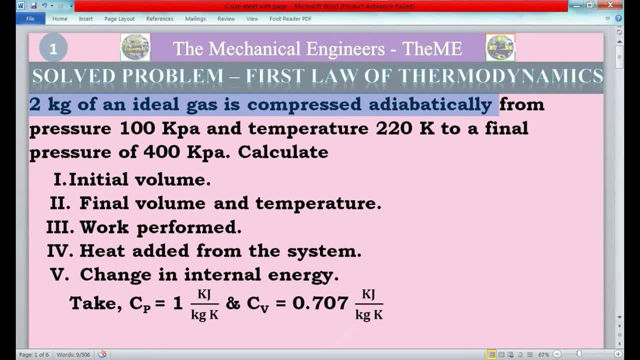 from the gas. The temperature and pressure of the gas will be increased. The volume of the gas will be decreased. So in this question the pressure of the gas is increased from 100 kilo Pascal to 400 kilo Pascal And the initial temperature of the gas is 220 Kelvin. 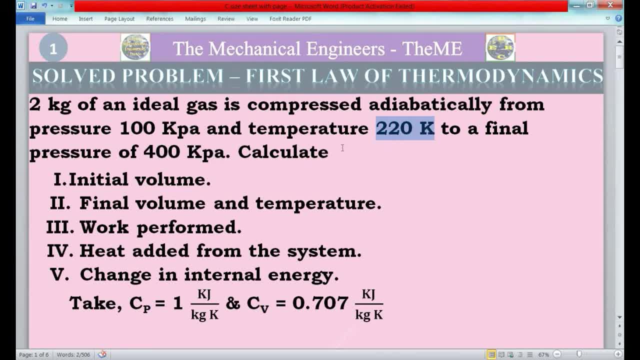 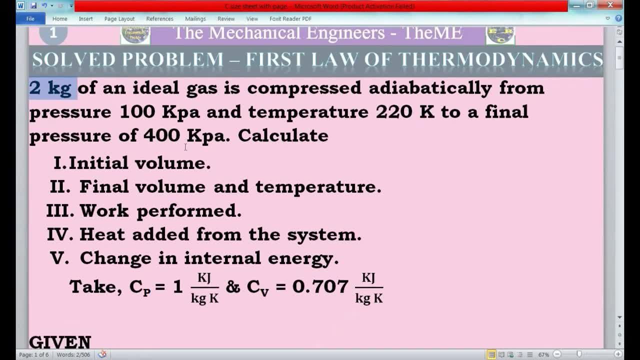 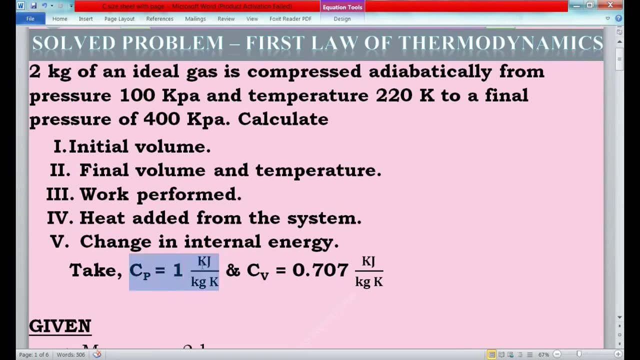 which means the temperature of the gas For compression process is 220 Kelvin and the mass of the gas is 2 kg. The specific heat added during constant pressure process is- Cp is equal to 1 kilo Joule per kg Kelvin, and the specific heat added during constant volume processes Cv, which is 0.707 kilo Joule. 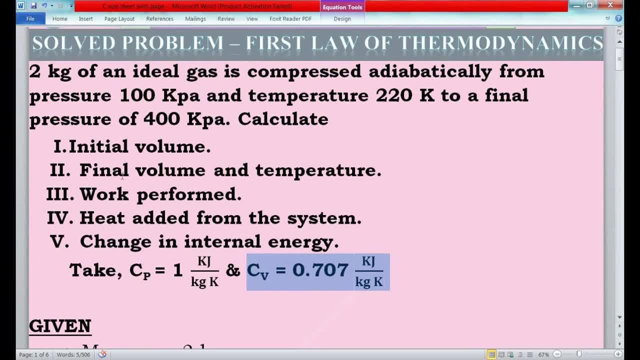 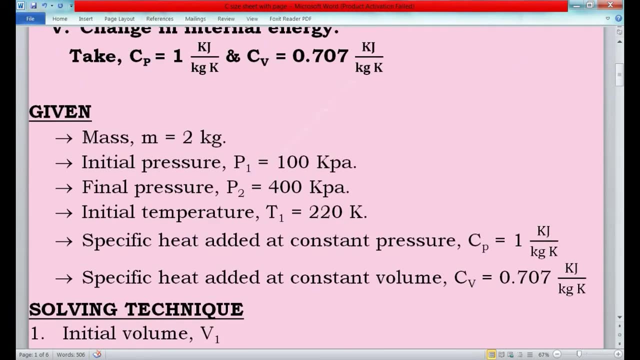 per kg Kelvin. So in this question we have to calculate the values of initial volume, final volume, temperature, work performed, heat added from the system and change in internal energy. next i will list out the given conditions from the question. first, mass of the gas is 2 kg, which is m the. 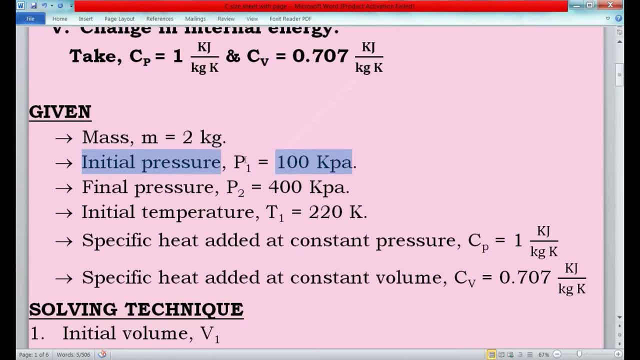 initial pressure of the gas is 100 kilo pascal, which is p1. the final pressure of the gas is 400 kilo pascal, which is p2. the initial temperature of the gas is 220 kelvin, which is t1. the specific heat added at constant pressure is 1 kilo joule per kg kelvin, which is cp. the specific heat added. 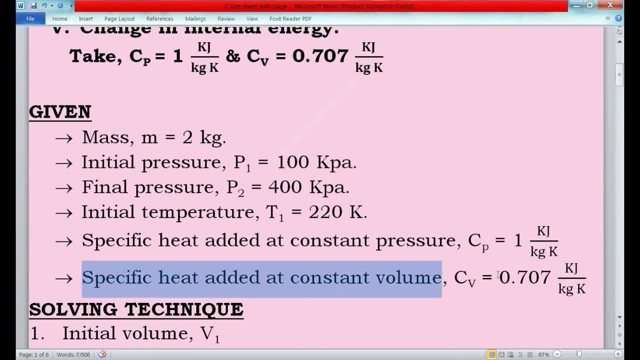 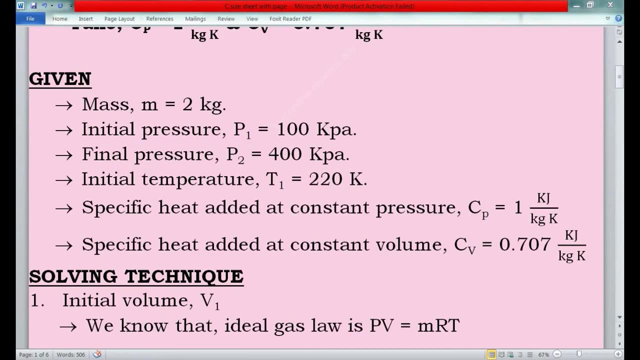 at constant volume is 0.707 kilo joule per kg kelvin, which is cv. so by using these six conditions i'm going to find the values of initial volume, final volume, final temperature, work performed, heat added from the system and change in internal energy. next is solving technique. we know that gas. 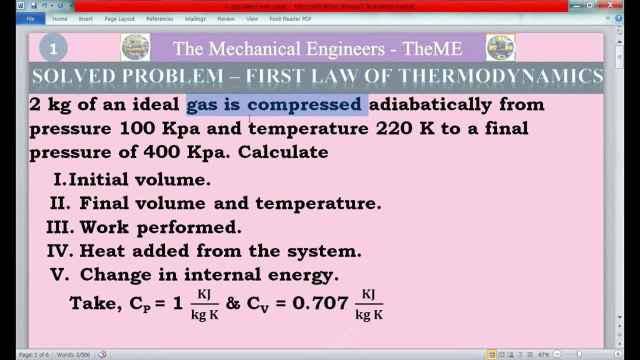 is being compressed, which means the gas is being compressed. the gas undergoes compression process. so during compression process the pressure of the gas will increase, the temperature of the gas will increase and the volume of the gas will decrease. to be precise, the initial pressure value in compression process will be lower. the final pressure value in 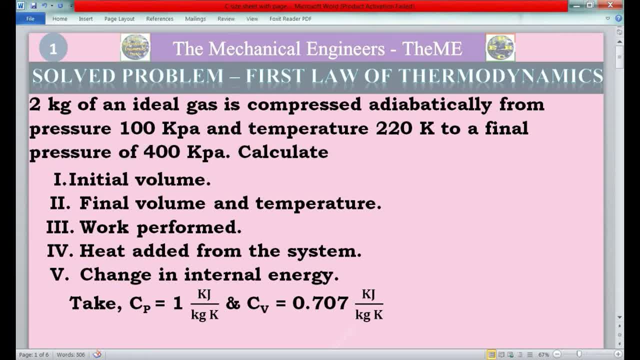 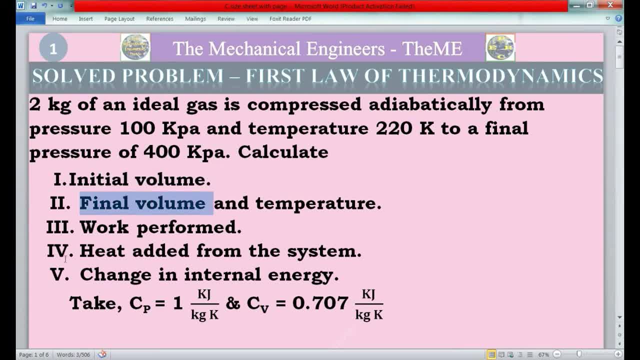 final temperature value in compression process will be higher. the final temperature value in compression process will be lower. final temperature value in compression process will be lower. the final temperature value in compression process will be lower. okay, so first we will find the value of initial. okay, so first we will find the value of initial. 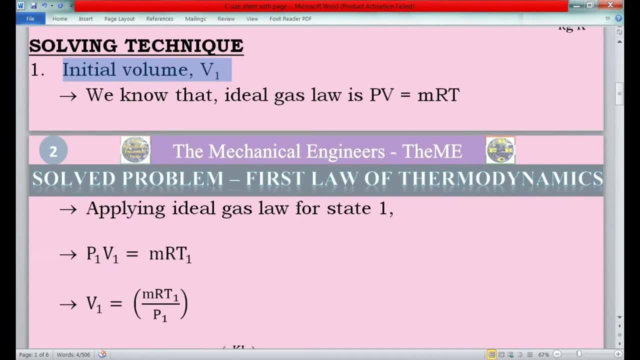 okay, so first we will find the value of initial volume, which is v1, for finding the value of volume, which is v1, for finding the value of volume, which is v1 for finding the value of initial volume. we are going to use the initial volume, we are going to use the. 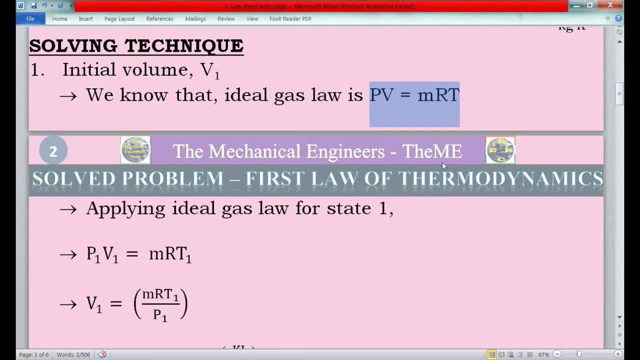 initial volume. we are going to use the formula of idle gas law, which is pv is formula of idle gas law, which is pv is formula of idle gas law which is pv is equal to mrt, equal to mrt, equal to mrt, where p is pressure, v is volume, m is mass. 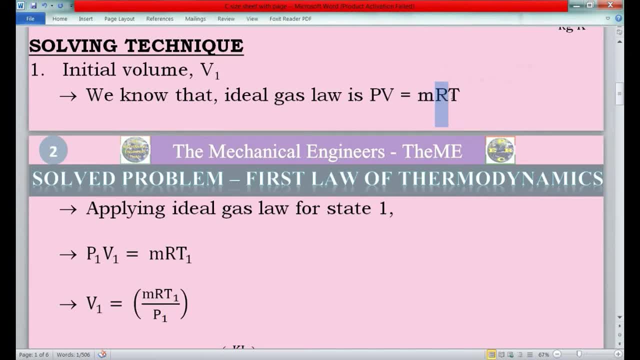 where p is pressure, v is volume, m is mass. where p is pressure, v is volume, m is mass. r is gas constant, which is 0.287. r is gas constant, which is 0.287. r is gas constant, which is 0.287 kilojoule per kg. kelvin and t is. 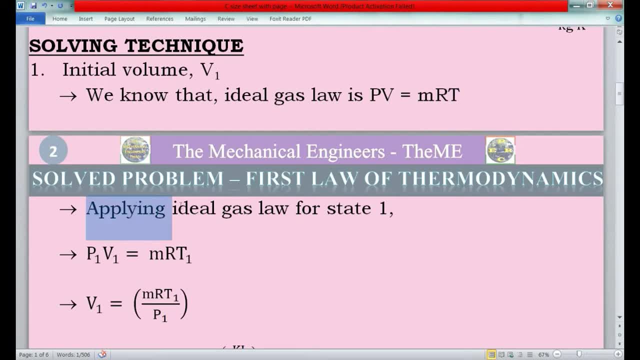 kilojoule per kg kelvin, and t is kilojoule per kg kelvin and t is temperature, temperature, temperature, okay, okay, okay. so now apply idle gas law on state 1. so now apply idle gas law on state 1. so now apply idle gas law on state 1. thereby this idle gas law equation will 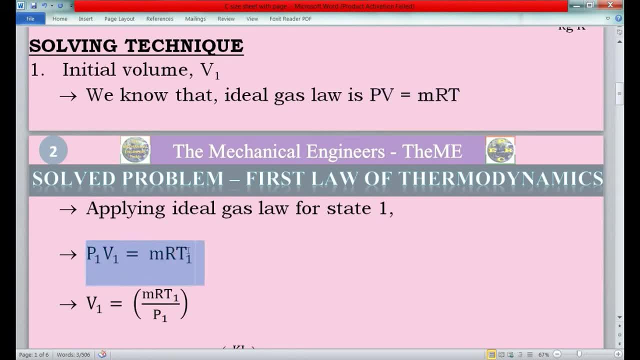 thereby this idle gas law equation will thereby this idle gas law equation will be rewritten as p1. v1 is equal to mrt1. be rewritten as p1. v1 is equal to mrt1. be rewritten as p1, v1 is equal to mrt1. so in this equation we know the values. 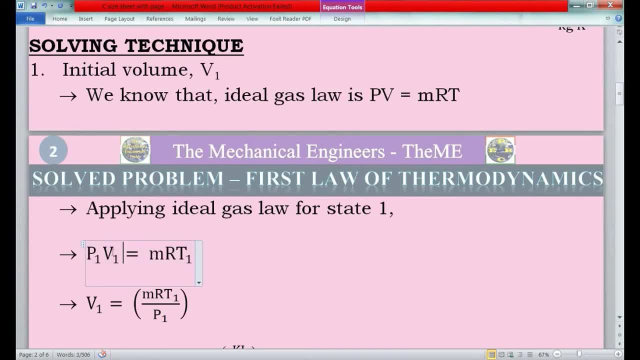 so in this equation we know the values. so in this equation we know the values of p1, m, r and t1. so we can easily find of p1, m, r and t1. so we can easily find of p1, m, r and t1. so we can easily find the value of v1. 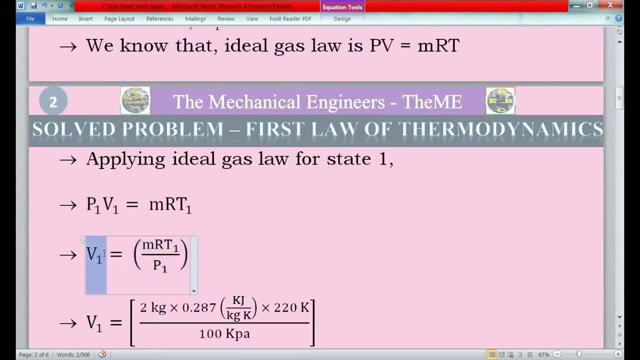 the value of v1. the value of v1. now bring this p1 to the oranges we get. now bring this p1 to the oranges we get. now bring this p1 to the oranges we get. v1 is equal to mrt1 divided by p1. 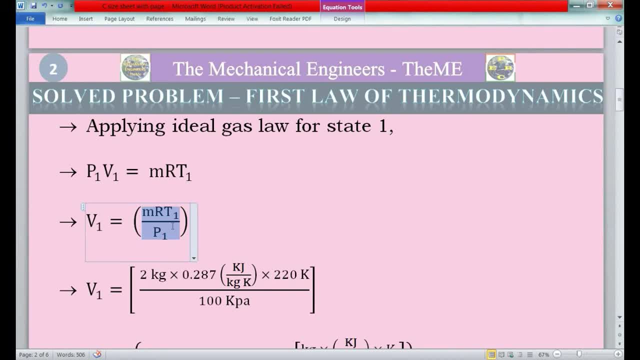 now substitute the values of m? r t1. and now substitute the values of m? r t1. and now substitute the values of m? r t1 and p1. in this formula p1, in this formula p1. in this formula we get: v1 is equal to 2 kg into 0.287. we get v1 is equal to 2 kg into 0.287. we get v1 is equal to 2 kg into 0.287. kilojoule per kg kelvin into 220 kelvin. kilojoule per kg kelvin into 220 kelvin. 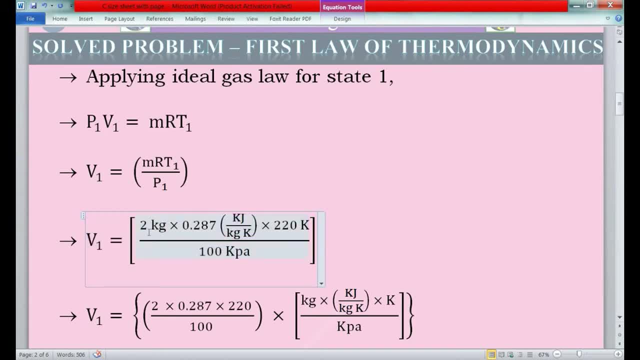 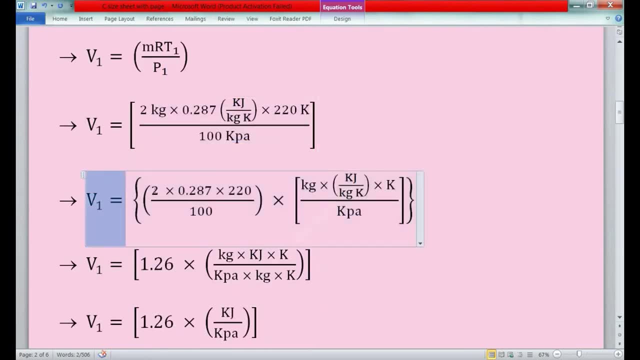 kilojoule per kg kelvin into 220 kelvin. divided. divided by 100 kilopascal in this oraches. split the numerical in this oraches. split the numerical in this oraches. split the numerical terms and s units, we get: v1 is equal to: 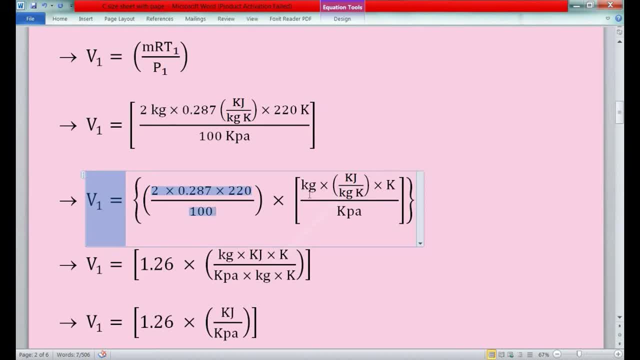 terms and s units, we get: v1 is equal to terms and s units. we get: v1 is equal to 2 into 0.287 into 220 divided by 100. 2 into 0.287 into 220 divided by 100. 2 into 0.287 into 220 divided by 100 into kg. into kilojoule per kg kelvin. 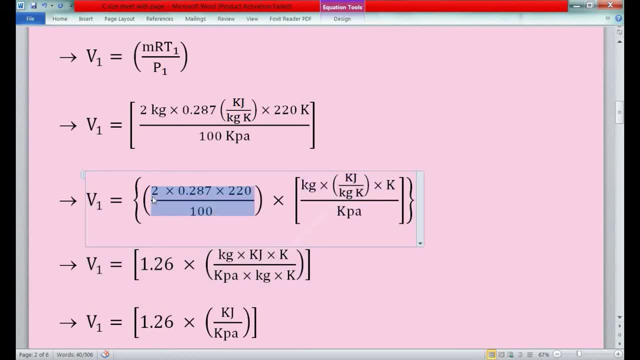 into kg. into kilojoule per kg kelvin. into kg. into kilojoule per kg kelvin into kelvin divided by kilo pascal into kelvin divided by kilo pascal into kelvin. divided by kilo pascal here 2 into 0.287. into 220 divided by 100. 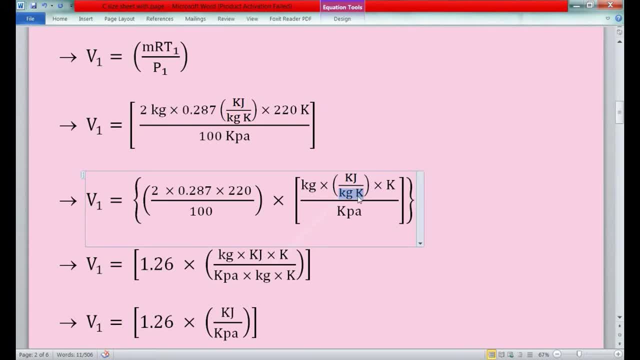 here 2 into 0.287. into 220 divided by 100. here 2 into 0.287 into 220 divided by 100 is 1.26, is 1.26, is 1.26. and bring this kg kelvin to the denominator. 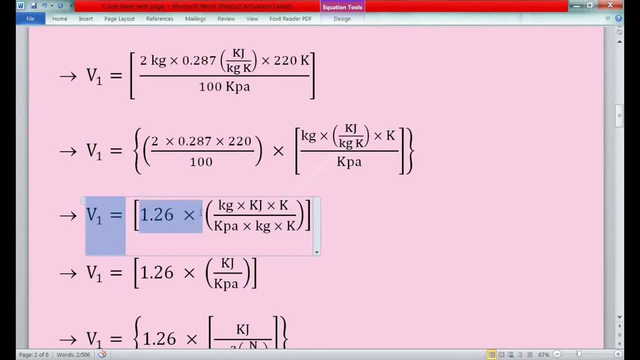 and bring this kg kelvin to the denominator. and bring this kg kelvin to the denominator. therefore, v1 is equal to 1.26 into kg. therefore, v1 is equal to 1.26 into kg. therefore, v1 is equal to 1.26 into kg into kilojoule, into kelvin, divided by: 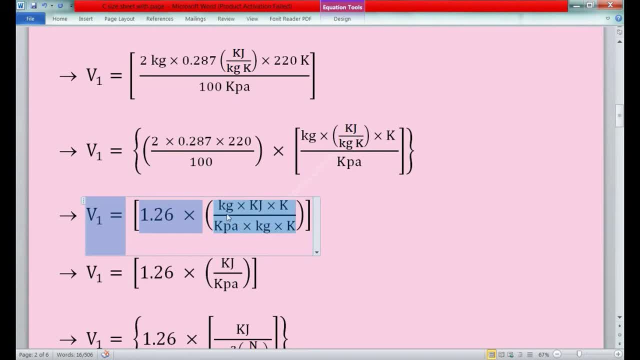 into kilojoule into kelvin. divided by into kilojoule into kelvin. divided by kilo pascal into kg into kelvin, kilo pascal into kg into kelvin, kilo pascal into kg into kelvin is kilojoule per kilo pascal. because 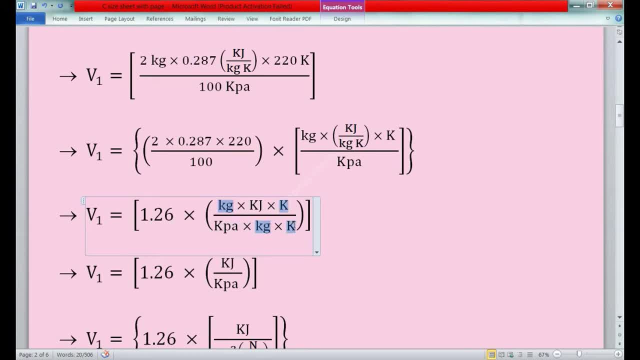 is kilojoule per kilo pascal. because is kilojoule per kilo pascal? because kg. kg gets cancelled and kelvin kelvin kg. kg gets cancelled and kelvin kelvin kg. kg gets cancelled and kelvin kelvin gets cancelled. 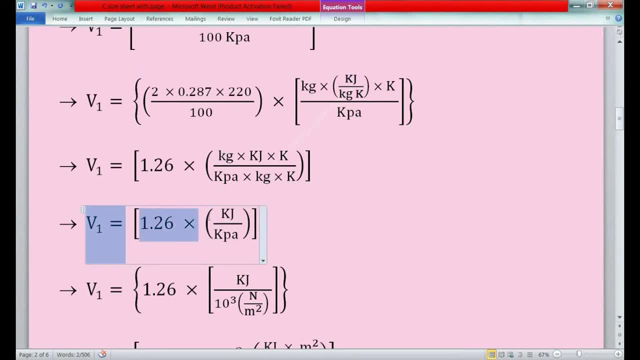 gets cancelled gets cancelled. therefore, v1 is equal to 1.26 into kilo. therefore, v1 is equal to 1.26 into kilo. therefore, v1 is equal to 1.26 into kilo joule per kilo pascal. joule per kilo pascal. 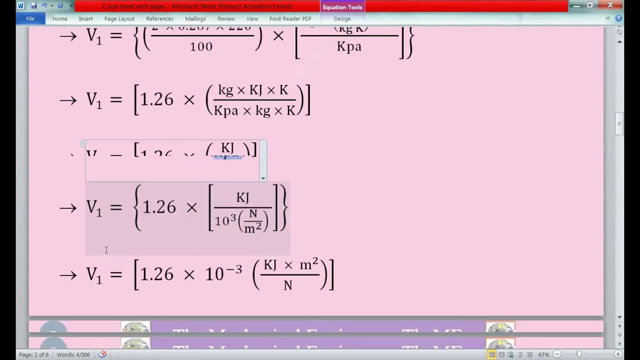 joule per kilo pascal. we know that kilo pascal is 10 power 3. we know that kilo pascal is 10 power 3. we know that kilo pascal is 10 power 3. newton per meter square. 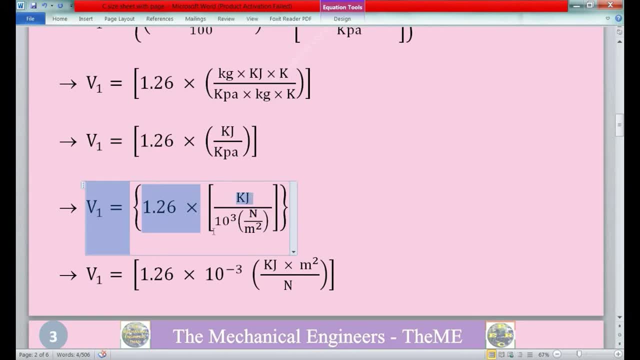 newton per meter square. newton per meter square, so v1 is equal to 1.26 into kilo joule, so v1 is equal to 1.26 into kilo joule, so v1 is equal to 1.26 into kilo joule per meter square. in this denominator, bring this: 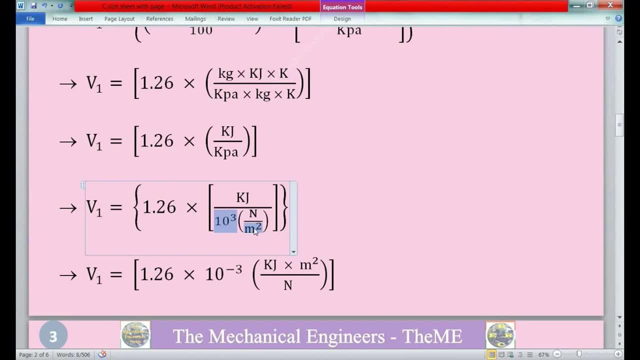 per meter square in this denominator. bring this per meter square in this denominator. bring this 10 power 3 and meter square to the 10 power 3 and meter square to the 10 power 3 and meter square to the numerator, we get. v1 is equal to 1.26. 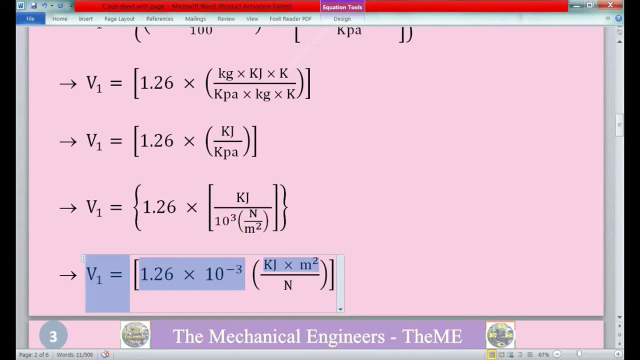 numerator: we get v1 is equal to 1.26. numerator: we get: v1 is equal to 1.26 into 10 power minus 3 into kilojoule. into 10 power minus 3 into kilo joule. into 10 power minus 3 into kilo joule. into meter square divided by newton. 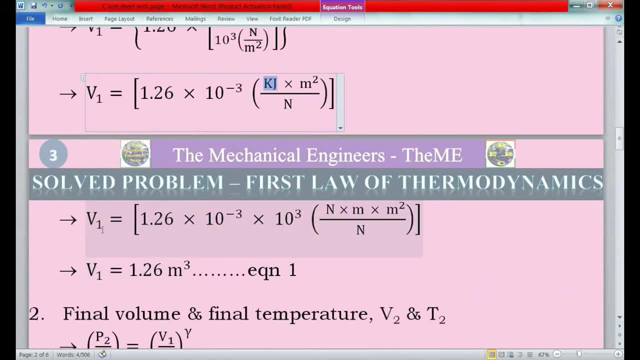 into meter square divided by newton. into meter square divided by newton. here kilo joule is 10 power 3 newton. here kilo joule is 10 power 3 newton. here kilo joule is 10 power 3 newton meter. therefore v1 is equal to 1.26. 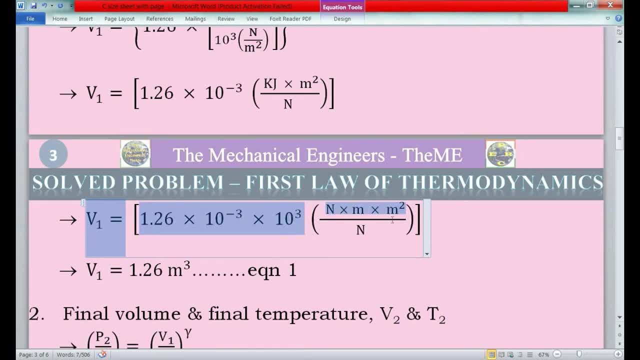 meter. therefore v1 is equal to 1.26 meter. therefore, v1 is equal to 1.26. into 10 power minus 3 into 10 power 3. into 10 power minus 3, into 10 power 3. into 10 power minus 3. into 10 power 3, into newton, into meter, into meter square. 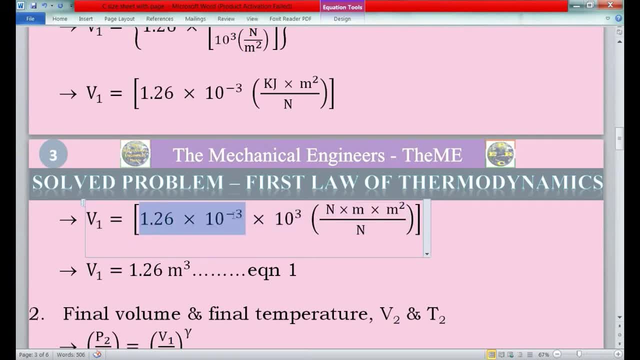 into newton, into meter, into meter square. into newton, into meter into meter square, divided by newton. divided by newton. divided by newton: here: 1.26 into 10, power minus 3 into 10, here 1.26 into 10, power minus 3 into 10. 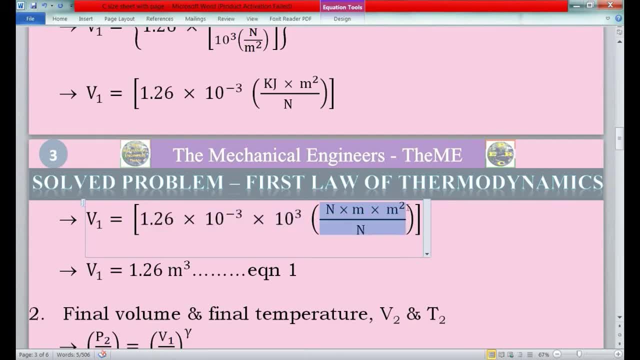 here 1.26 into 10. power minus 3 into 10, power 3 is 1.26, power 3 is 1.26, power 3 is 1.26. and newton into meter into meter square. and newton into meter into meter square. 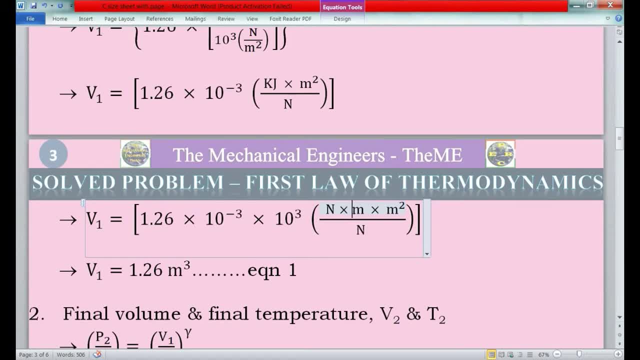 and newton into meter, into meter. square divided by newton is divided by newton, is divided by newton, is meter meter cube because newton, newton meter, meter cube because newton, newton meter cube because newton, newton gets cancelled and meter into meter. 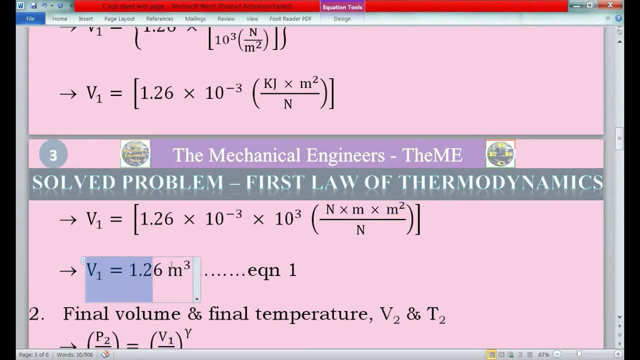 gets cancelled and meter into meter gets cancelled and meter into meter. square is meter cube, so v1 is equal to square is meter cube, so v1 is equal to square. is meter cube, so v1 is equal to 1.26 meter cube. consider this one as: 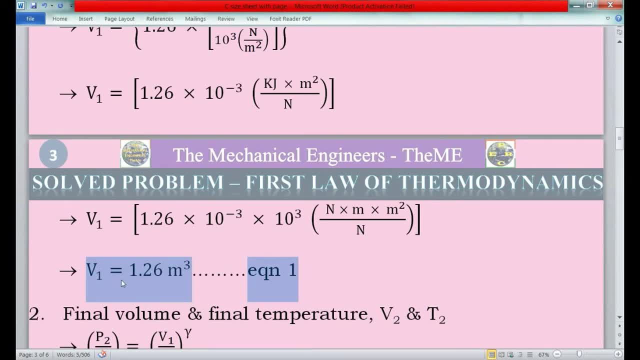 1.26 meter cube. consider this one as 1.26 meter cube. consider this one as equation 1. so the initial volume value, equation 1. so the initial volume value, equation 1. so the initial volume value of gas is 1.26 meter cube. 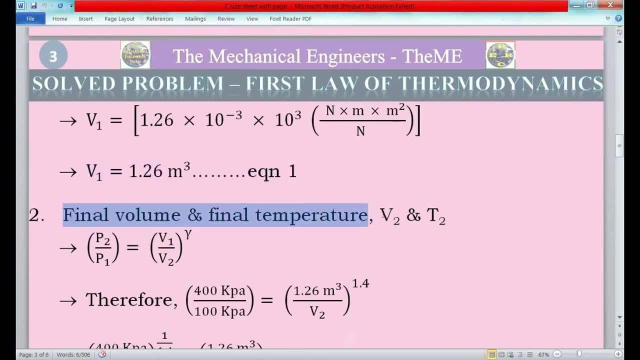 of gas is 1.26 meter cube of gas is 1.26 meter cube. next we will find the values of final. next we will find the values of final. next we will find the values of final volume and final temperature. volume and final temperature. volume and final temperature, which is v2 and t2. remember, 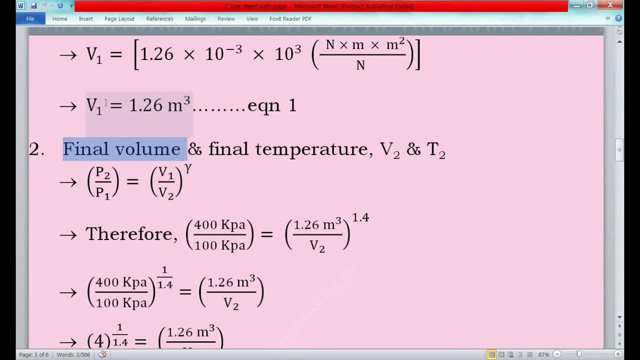 which is v2 and t2. remember which is v2 and t2. remember the final volume value should be less. the final volume value should be less. the final volume value should be less than the initial volume value 1.26 meter. than the initial volume value 1.26 meter. 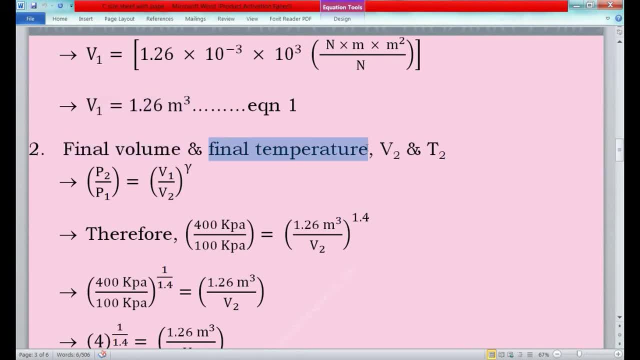 than the initial volume value: 1.26 meter cube. and the final temperature value: cube. and the final temperature value cube. and the final temperature value should be more than the initial. should be more than the initial. should be more than the initial temperature value: 220 kelvin. 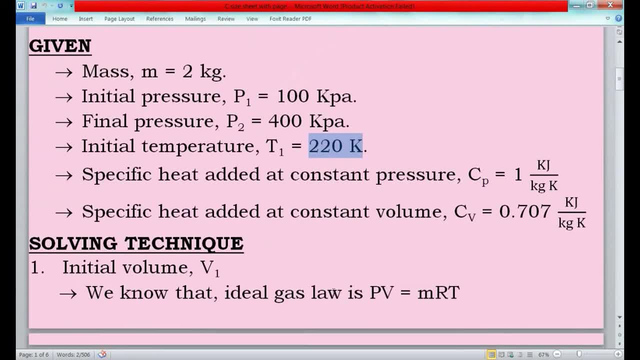 temperature value: 220 kelvin. temperature value: 220 kelvin. okay, so first we will find the value of: okay, so first we will find the value of. okay, so first we will find the value of final volume, final volume, final volume. we know that the compression of gas is. 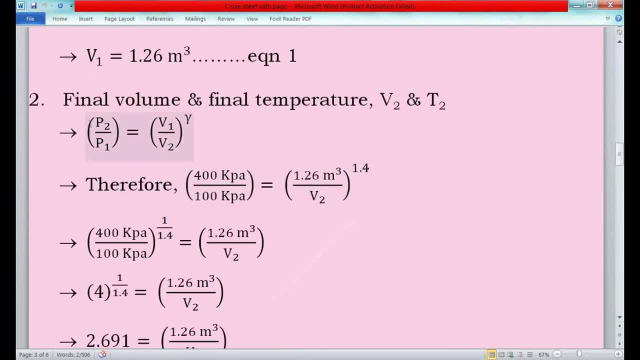 we know that the compression of gas is, we know that the compression of gas is carried out during adiabatic process, carried out during adiabatic process, carried out during adiabatic process. so the universal formula for compression, so the universal formula for compression. 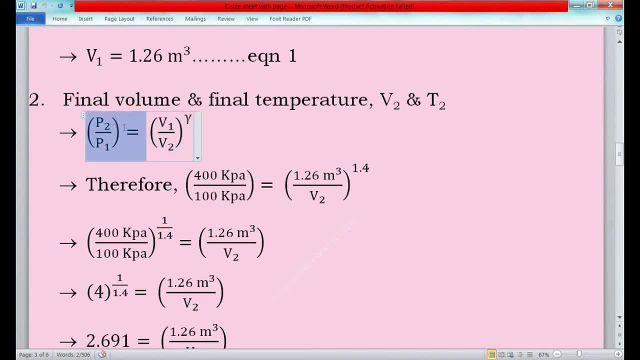 so the universal formula for compression during adiabatic process is given by: during adiabatic process, is given by: during adiabatic process. is given by p2 by p1 is equal to v1 by v2. p2 by p1 is equal to v1 by v2. 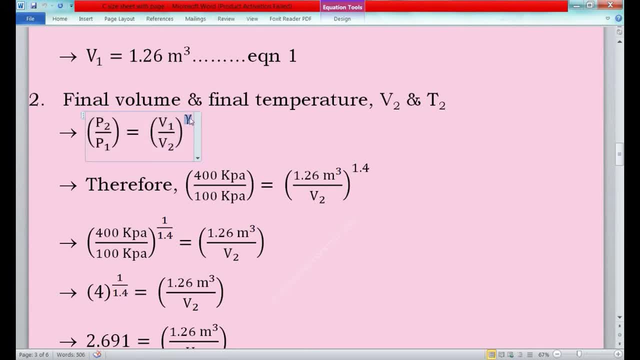 p2 by p1 is equal to v1 by v2. v1 by v2 to the power of gamma. where gamma v1 by v2 to the power of gamma. where gamma v1 by v2 to the power of gamma. where gamma is adiabatic constant. 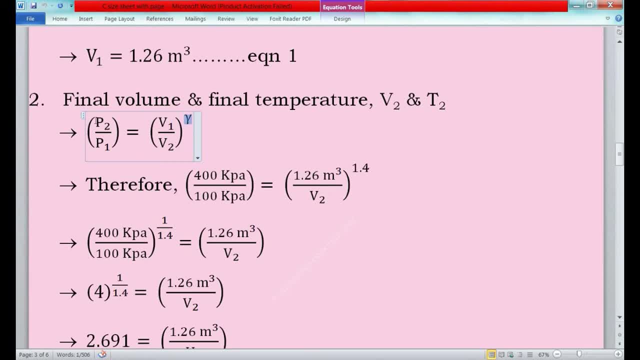 is adiabatic constant is adiabatic constant and the universal value is 1.4. so in this and the universal value is 1.4. so in this and the universal value is 1.4. so in this formula, we know the values of p2. 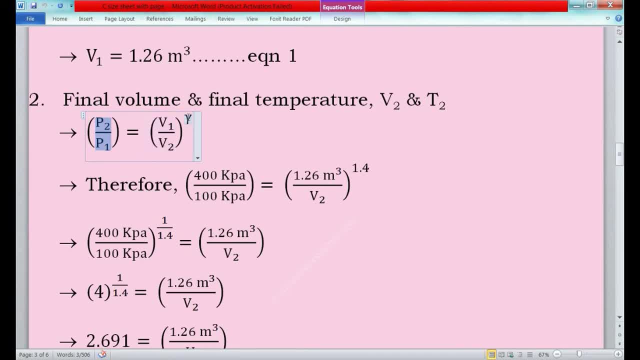 formula. we know the values of p2 formula. we know the values of p2, p1, v1 and gamma. so just substitute the p1, v1 and gamma. so just substitute the p1, v1 and gamma. so just substitute the values in this formula. values in this formula. 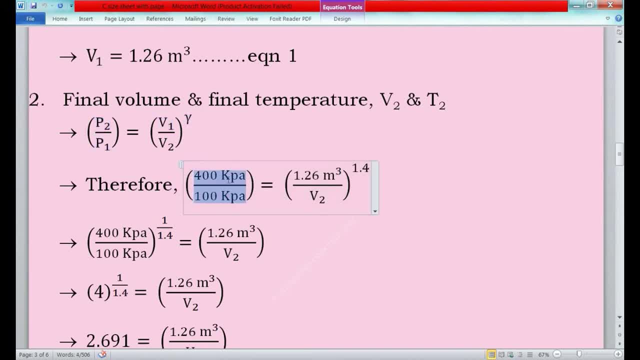 values. in this formula, we get 400 kilopascal divided by 100. we get 400 kilopascal divided by 100. we get 400 kilopascal divided by 100. kilopascal is equal to. kilopascal is equal to. kilopascal is equal to 1.26 meter cube divided by v2 to the 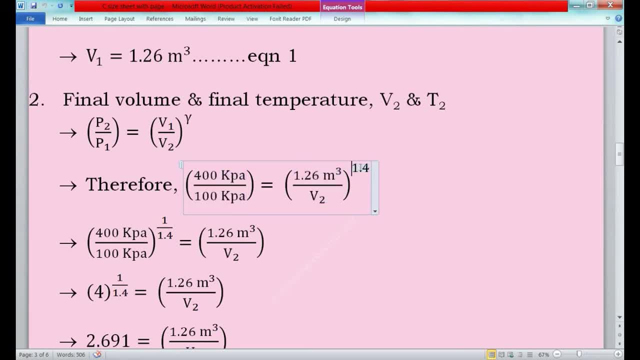 1.26 meter cube divided by v2 to the 1.26 meter cube divided by v2 to the power of 1.4. power of 1.4, power of 1.4. now bring this 1.4 to the lhs, we get 400. 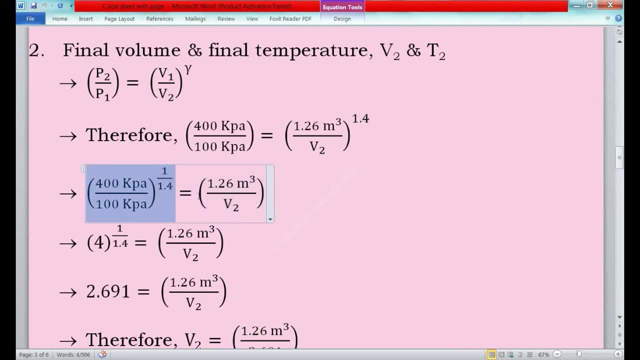 now bring this 1.4 to the lhs, we get 400. now bring this 1.4 to the lhs, we get 400 kilopascal divided by 100 kilopascal to kilopascal. divided by 100 kilopascal to kilopascal. divided by 100 kilopascal to the power of 1, divided by 1.4 is equal. 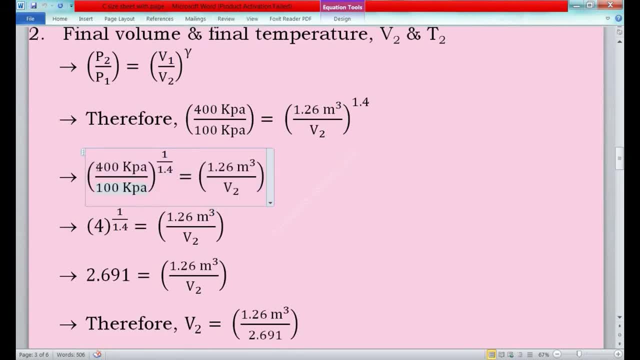 the power of 1 divided by 1.4 is equal. the power of 1 divided by 1.4 is equal to 1.26 meter cube divided by v2 to 1.26 meter cube divided by v2 to 1.26 meter cube divided by v2, so 400 kilopascal divided by 100. 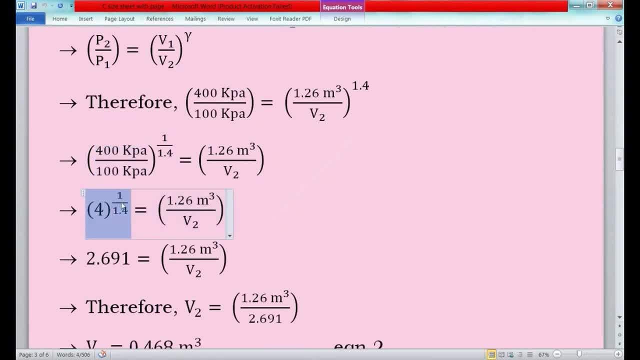 so 400 kilopascal divided by 100. so 400 kilopascal divided by 100 kilopascal is 4. therefore, 4 to the power, kilopascal is 4, therefore 4 to the power. kilopascal is 4, therefore 4 to the power of 1 by 1.4 is equal to 1.26 meter cube. of 1 by 1.4 is equal to 1.26 meter. cube of 1 by 1.4 is equal to 1.26 meter cube. divided by v2. here 4 to the power of 1. divided by 1.4 is equal to 1.26 meter cube. divided by v2. here 4 to the power of 1. 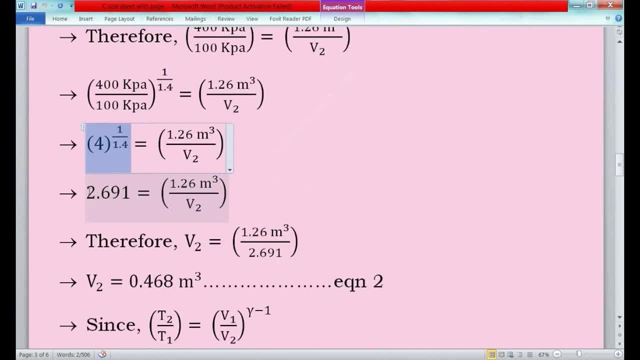 divided by 1.4 is equal to 1.26 meter cube divided by v2. here 4 to the power of 1 divided by 1.4. is divided by 1.4. is divided by 1.4 is 2.691. therefore, 2.691 is equal to. 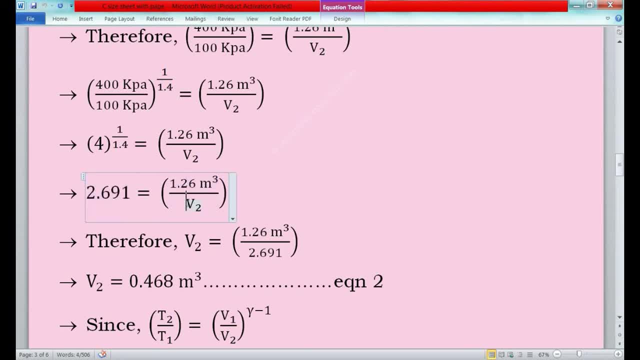 2.691. therefore, 2.691 is equal to 2.691. therefore, 2.691 is equal to 1.26 meter cube divided by v2. 1.26 meter cube divided by v2. 1.26 meter cube divided by v2. so here, bring this v2 to the lhs and. 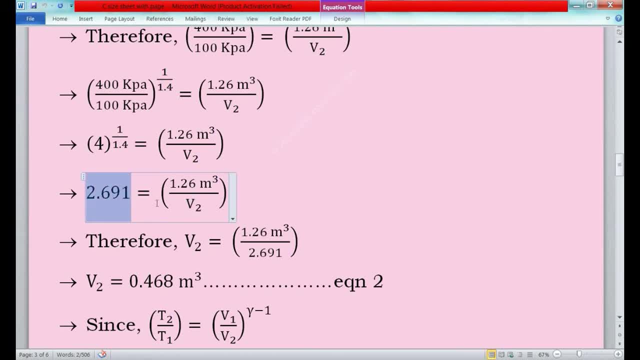 so here, bring this v2 to the lhs. and so here, bring this v2 to the lhs and move this, move this, move this now: 2.69, 2.691 to the arches we get now 2.69, 2.691 to the arches we get. 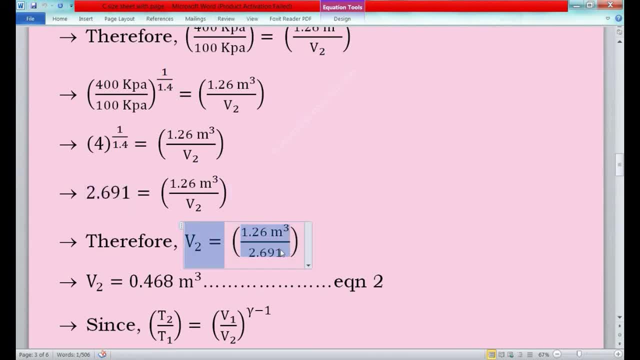 now 2.69, 2.691 to the arches we get. v2 is equal to 1.26 meter cube divided by v2 is equal to 1.26 meter cube divided by v2 is equal to 1.26 meter cube divided by 2.691. 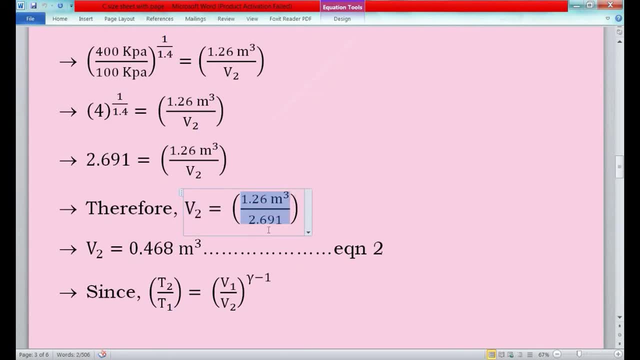 2.691, 2.691 here. 1.26 meter cube divided by 2.691 is here: 1.26 meter cube divided by 2.691 is here: 1.26 meter cube divided by 2.691 is 0.468 meter cube. therefore v2 is: 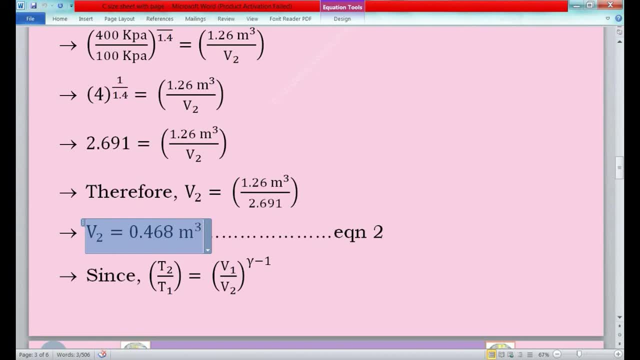 0.468 meter cube. therefore, v2 is 0.468 meter cube. therefore, v2 is: v2 is equal to 0.468 meter cube. v2 is equal to 0.468 meter cube. v2 is equal to 0.468 meter cube and consider this one as equation 2, so v2. 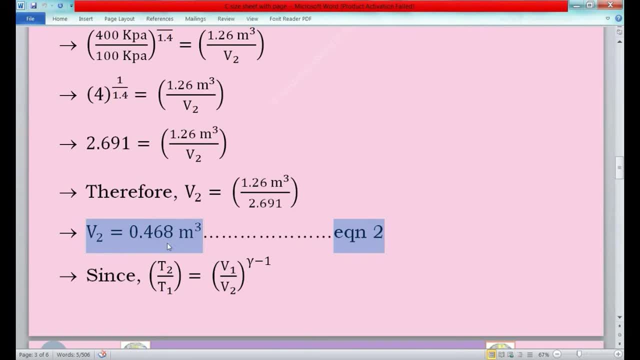 and consider this one as equation 2, so v2. and consider this one as equation 2, so v2 is equal to 0.468 meter cube. is is equal to 0.468 meter cube. is is equal to 0.468 meter cube is nothing but the final volume value of. 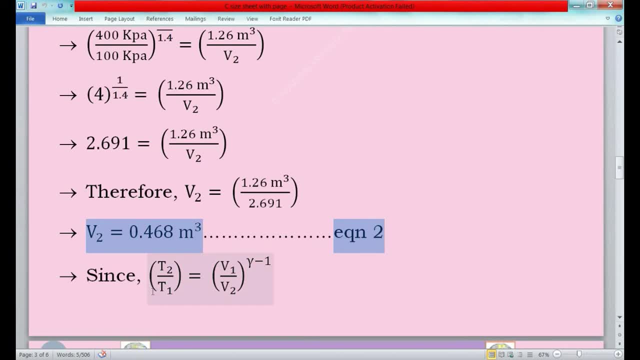 nothing but the final volume value of nothing, but the final volume value of gas, gas, gas. now we will find the value of final, now we will find the value of final, now we will find the value of final temperature, temperature, temperature. there is another universal formula for. there is another universal formula for. 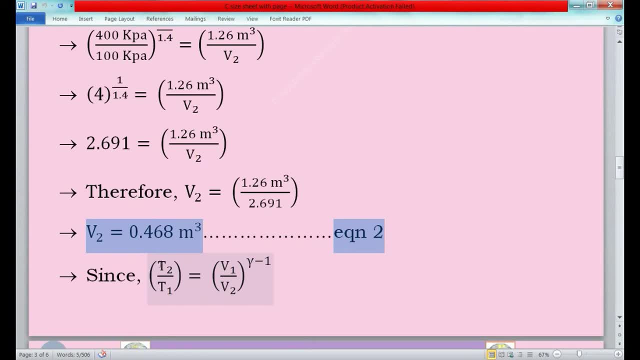 there is another universal formula for compression during adiabatic process: compression during adiabatic process, compression during adiabatic process, and the formula is: and the formula is: and the formula is: t2 by t1 is equal to v1 by v2 to the. 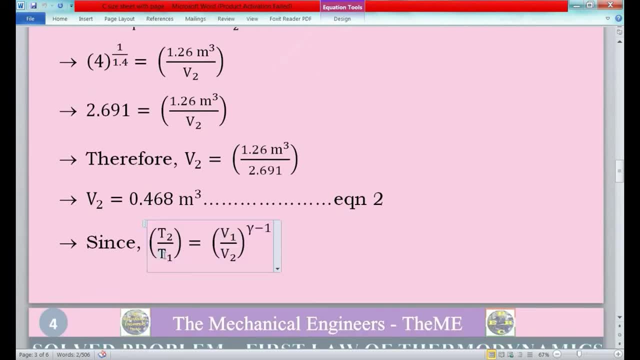 t2 by t1 is equal to v1 by v2 to the t2 by t1 is equal to v1 by v2 to the power of gamma minus one. power of gamma minus one. power of gamma minus one. okay, so in this formula, bring this t1 to: 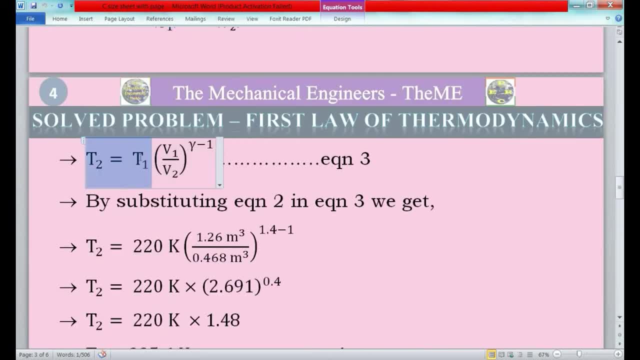 okay. so in this formula, bring this t1 to: okay. so in this formula, bring this t1 to the arches, the arches, the arches. we get t2 is equal to t1 into v1 by v2. we get t2 is equal to t1 into v1 by v2. 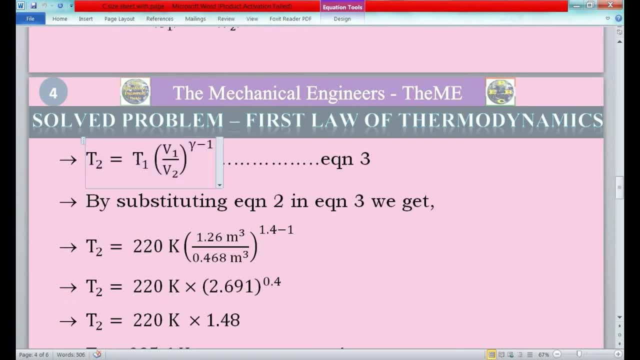 we get t2 is equal to t1- into v1 by v2 to the power of gamma minus one, to the power of gamma minus one to the power of gamma minus one. so in this formula we know the values of. so in this formula we know the values of. 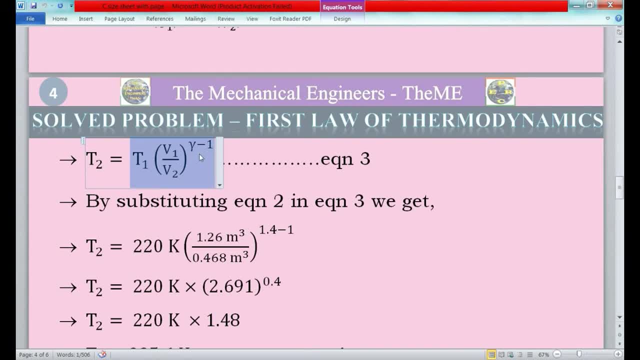 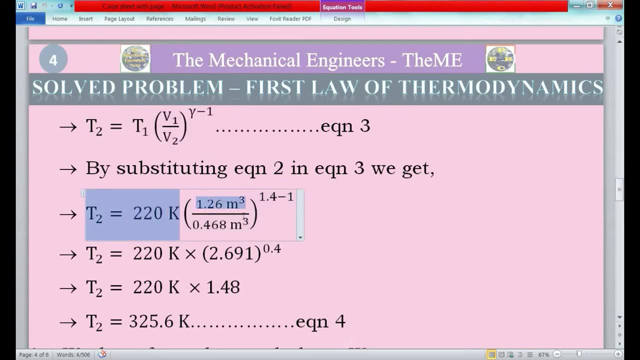 so in this formula we know the values of t1, v1, v2 and gamma. so so just substitute t1, v1, v2 and gamma. so so just substitute t1, v1, v2 and gamma. so so just substitute the values, the values, the values we get. t2 is equal to 220 kelvin into 1.26. we get t2 is equal to 220 kelvin into 1.26. we get t2 is equal to 220 kelvin into 1.26 meter cube divided by 0.468 meter cube to meter cube divided by 0.468 meter cube to. 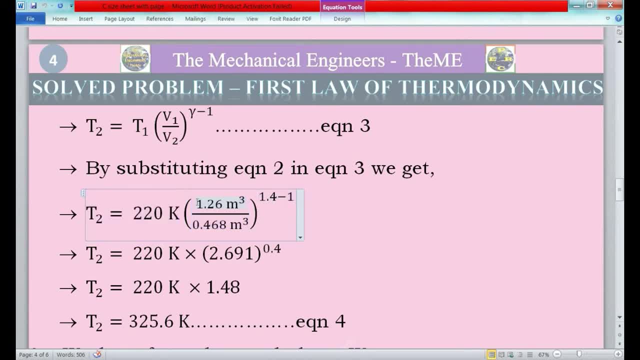 meter cube divided by 0.468 meter cube, to the power of 1.4 minus 1.. the power of 1.4 minus 1.. the power of 1.4 minus 1.. so here, 1.26 meter cube divided by 0.468. 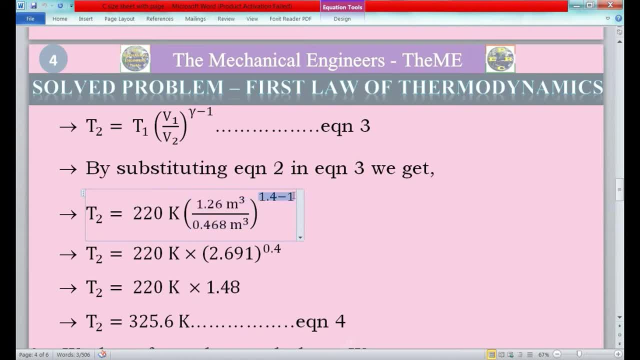 so here 1.26 meter cube divided by 0.468. so here 1.26 meter cube divided by 0.468. meter cube is 2.691, and 1.4 minus 1 is. meter cube is 2.691, and 1.4 minus 1 is: 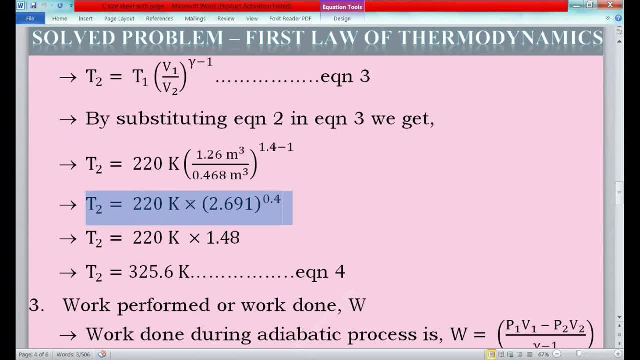 meter cube is 2.691 and 1.4 minus 1 is 0.4. therefore t2 is equal to 220 kelvin 0.4. therefore t2 is equal to 220 kelvin 0.4. therefore t2 is equal to 220 kelvin into 2.691 to the power of 0.4. into 2.691 to the power of 0.4 into 2.691 to the power of 0.4. here 2.691 to the power of 0.4 is. here 2.691 to the power of 0.4 is. 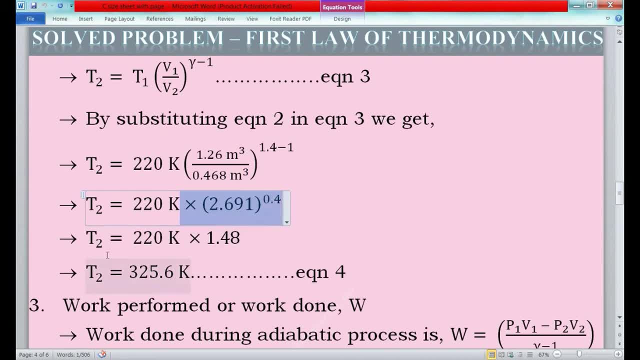 here 2.691 to the power of 0.4 is 1.48. therefore t2 is equal to 1.48. therefore t2 is equal to 1.48. therefore t2 is equal to 220 kelvin into 1.48. 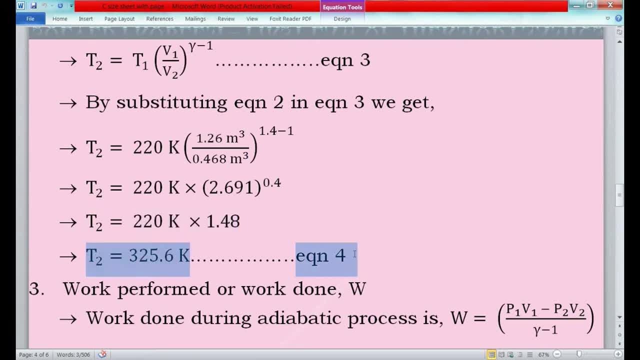 220 kelvin into 1.48, so t2 is 325.6 kelvin. and consider this so t2 is 325.6 kelvin. and consider this, so t2 is 325.6 kelvin. and consider this one as equation 4, so the final. 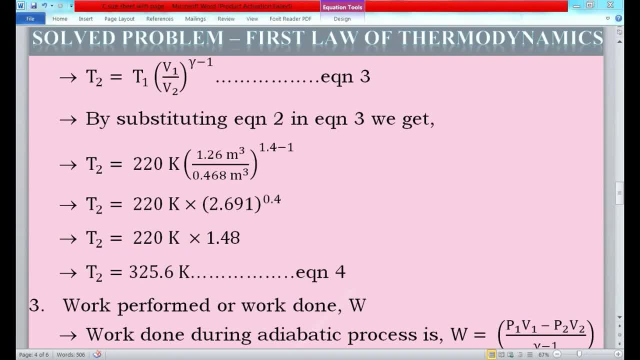 one as equation 4. so the final one as equation 4. so the final temperature value of gas is 325.6 kelvin. temperature value of gas is 325.6 kelvin. temperature value of gas is 325.6 kelvin. next we will find the value of work done. 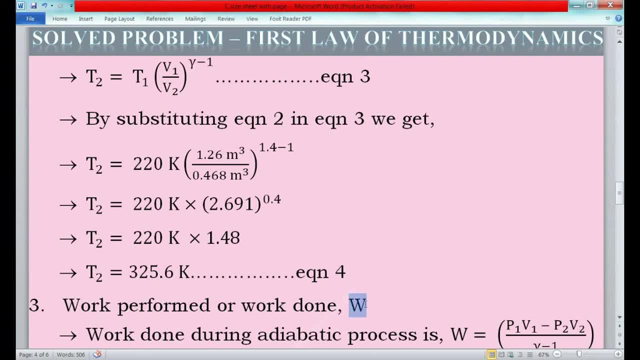 next, we will find the value of work done. next, we will find the value of work done or work performed which is taken as w, or work performed which is taken as w or work performed which is taken as w. so the universal formula for compression, so the universal formula for compression. 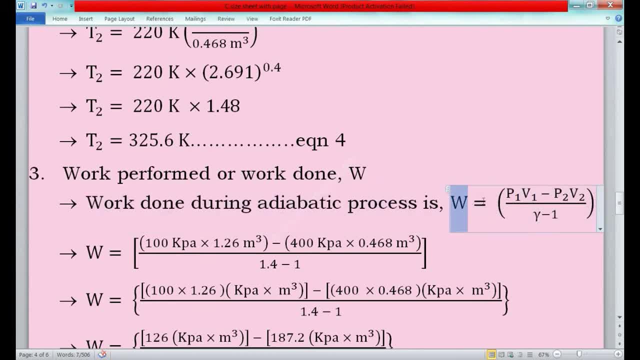 so the universal formula for compression work during adiabatic process is given. work during adiabatic process is given. work during adiabatic process is given. by w is equal to p1 v1 minus p2 v2. by w is equal to p1 v1 minus p2 v2. 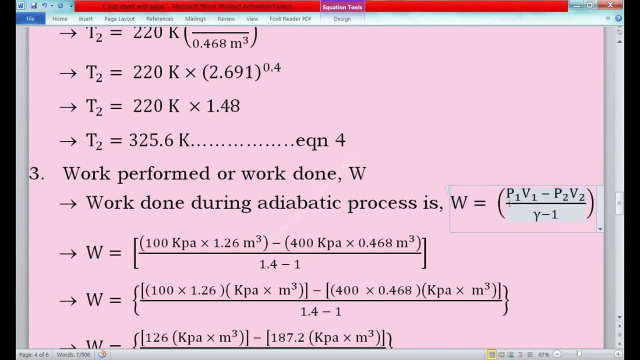 by w is equal to p1, v1 minus p2, v2 divided by gamma minus 1, divided by gamma minus 1, divided by gamma minus 1. so in this formula we know the values of. so in this formula we know the values of. so in this formula we know the values of p1, v1, p2, v2 and gamma. so we can easily. 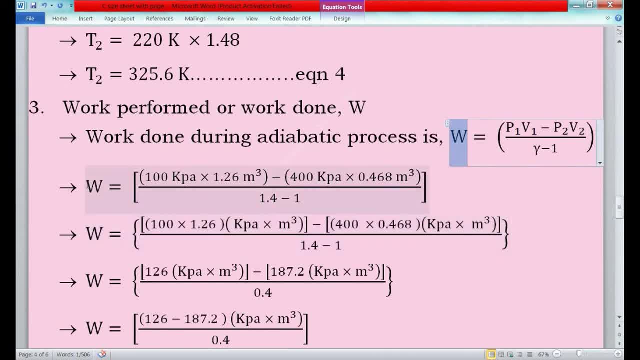 p1, v1, p2, v2 and gamma. so we can easily p1, v1, p2, v2 and gamma. so we can easily find the value of work done. find the value of work done. find the value of work done. so just substitute the values. we get w. 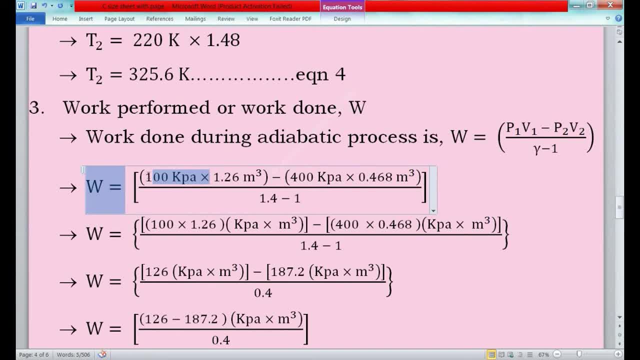 so just substitute the values. we get w. so just substitute the values we get. w is equal to 100 kilopascal into 1.26 is equal to 100 kilopascal into 1.26 is equal to 100 kilopascal into 1.26 meter cube minus 400 kilopascal into. 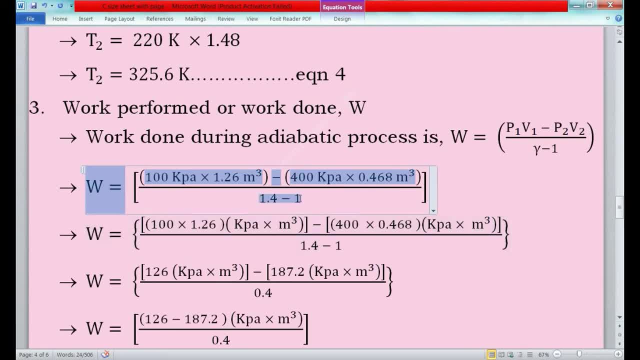 meter cube minus 400 kilopascal into meter cube minus 400 kilopascal. into 0.468 meter cube divided by 1.4 minus 1. 0.468 meter cube divided by 1.4 minus 1. 0.468 meter cube divided by 1.4 minus 1. in this orages split the numerical terms. 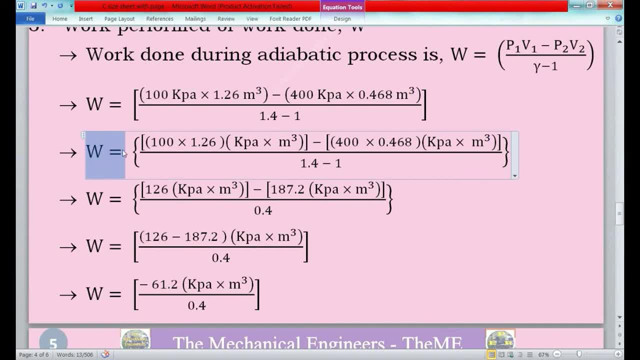 in this orages, split the numerical terms. in this orages, split the numerical terms and s units we get. and s units we get. and s units we get. w is equal to 100 into 1.26 into. w is equal to 100 into 1.26 into. 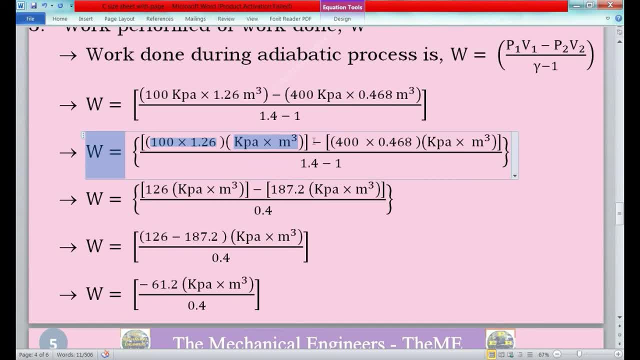 w is equal to 100 into 1.26 into kilopascal into meter cube, minus 400 kilopascal into meter cube, minus 400 kilopascal into meter cube, minus 400 into 0.468 into kilopascal into meter cube. 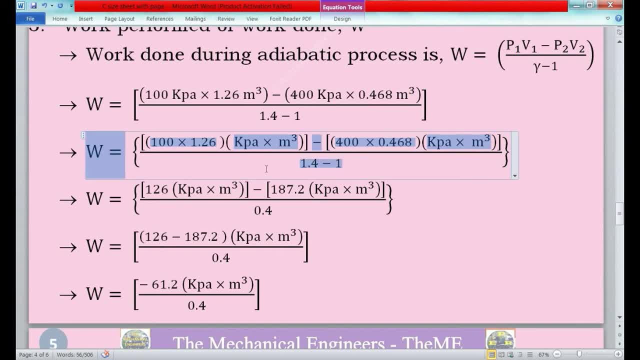 into kilopascal, into meter cube whole divided by 1.4 minus 1 whole. divided by 1.4 minus 1 whole. divided by 1.4 minus 1. here: 100 into 1.26 is 126. here: 100 into 1.26 is 126. 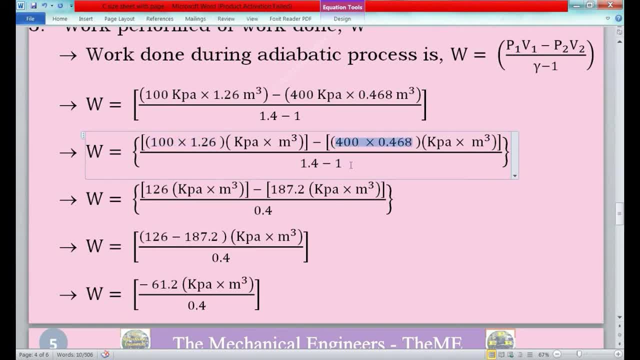 here: 100 into 1.26 is 126, and 400 into 0.468 is 187.2, and 400 into 0.468 is 187.2, and 400 into 0.468 is 187.2, and 1.4 minus 1 is 0.4. therefore w is. 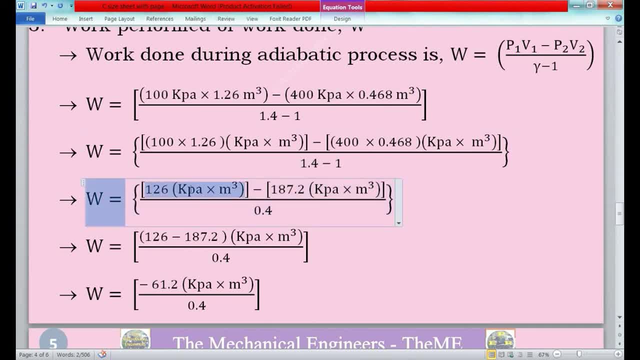 and 1.4 minus 1 is 0.4, therefore w is: and 1.4 minus 1 is 0.4. therefore w is equal to, equal to: equal to 126 into kilopascal into meter cube. 126 into kilopascal into meter cube. 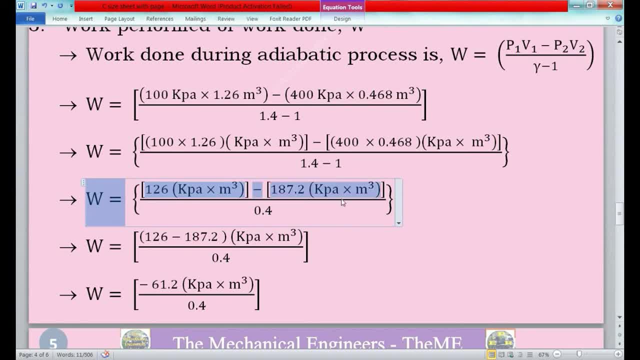 126 into kilopascal into meter cube minus 187.2. into kilopascal into meter minus 187.2. into kilopascal into meter minus 187.2. into kilopascal into meter cube divided by 0.4. cube divided by 0.4. 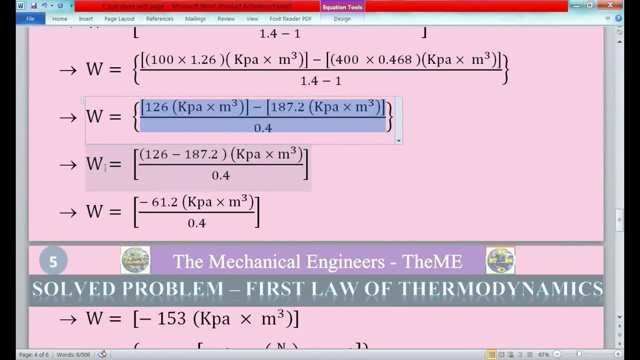 cube divided by 0.4 in this rhs split the numerical terms in this rhs split. the numerical terms in this rhs split the numerical terms and s units we get w is equal to 126 and s units we get w is equal to 126 and s units we get w is equal to 126 minus 187.2 into kilopascal. into meter. 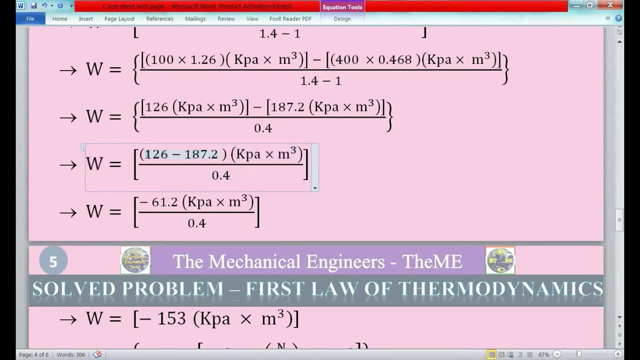 minus 187.2 into kilopascal into meter minus 187.2, into kilopascal, into meter cube divided by 0.4 cube, divided by 0.4 cube, divided by 0.4, so here 126 minus 187.2 is: 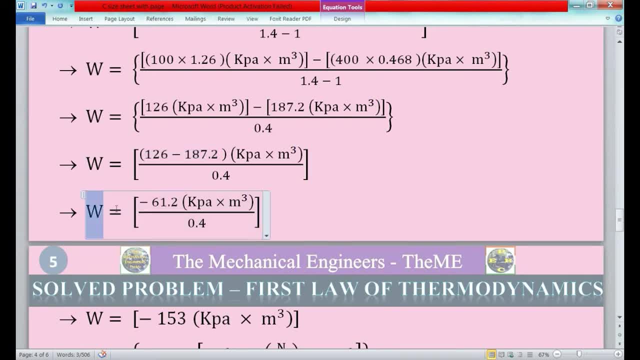 so here 126 minus 187.2 is. so here 126 minus 187.2 is minus 61.2. therefore w is equal to minus 61.2. therefore w is equal to minus 61.2. therefore w is equal to minus 161.2. into kilopascal, into meter: 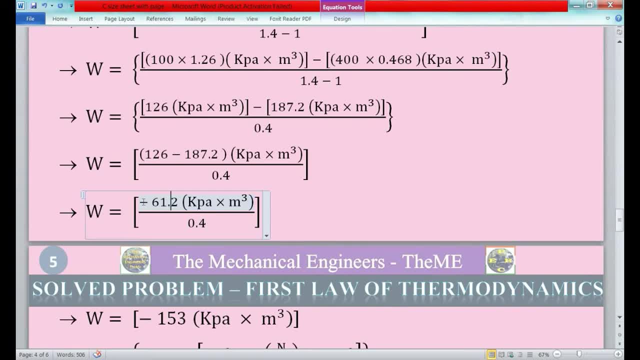 minus 161.2 into kilopascal into meter. minus 161.2 into kilopascal into meter cube divided by 0.4 cube divided by 0.4 cube divided by 0.4. here, minus 61.2 divided by 0.4 is: 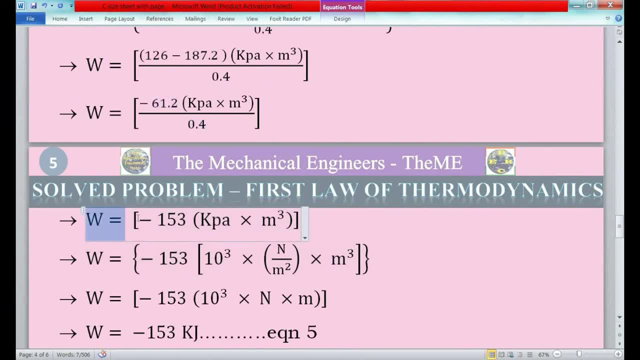 here minus 61.2 divided by 0.4 is here: minus 61.2 divided by 0.4 is minus 153. therefore, w is equal to minus 153. therefore, w is equal to minus 153. therefore, w is equal to minus 153. into kilopascal, into meter cube. 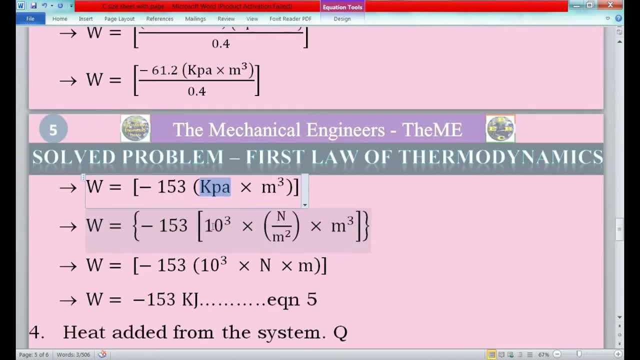 minus 153 into kilopascal into meter cube, minus 153 into kilopascal into meter cube. we know that kilopascal is 10 power 3. we know that kilopascal is 10 power 3. we know that kilopascal is 10 power 3 newton per meter square. therefore, w is: 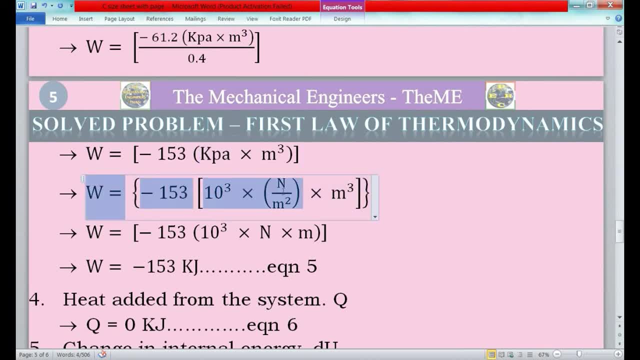 newton per meter square. therefore w is newton per meter square. therefore, w is equal to minus 153 into 10 power 3, into equal to minus 153 into 10 power 3, into equal to minus 153 into 10 power 3, into newton per meter square, into meter cube. 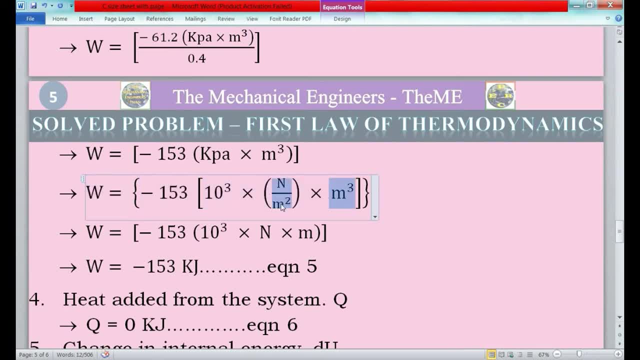 newton per meter square into meter cube. newton per meter square into meter cube. here newton per meter square into meter. here newton per meter square into meter. here newton per meter square into meter cube is cube, is cube, is newton meter, because meter square and 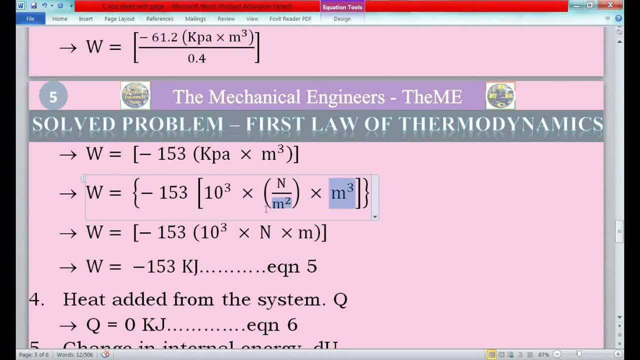 newton meter because meter square and newton meter because meter square and meter cube gets cancelled. therefore meter meter cube gets cancelled. therefore meter meter cube gets cancelled. therefore, meter will be, the will be, the will be the remaining term. okay, so w is equal to remaining term. okay, so w is equal to. 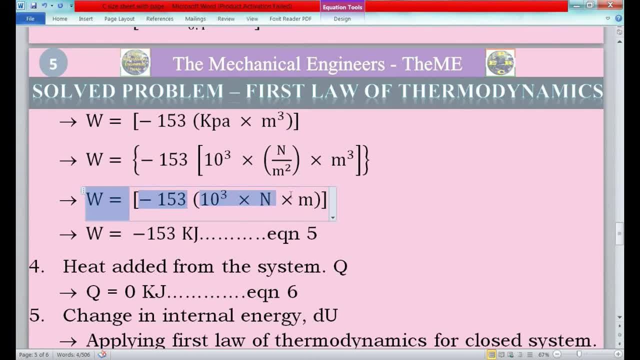 remaining term. okay, so w is equal to minus 153 into 10 power 3 into newton, minus 153 into 10 power 3 into newton. minus 153 into 10 power 3 into newton into meter. we know that 10 power 3 into. 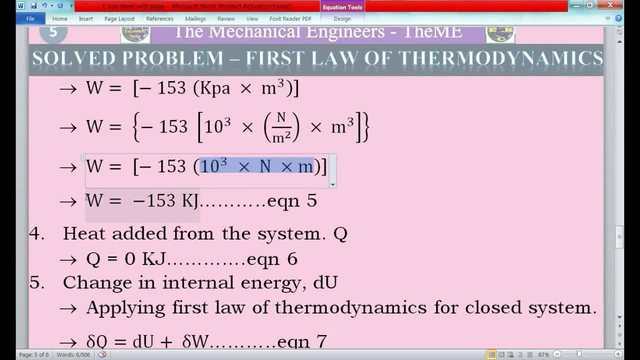 into meter. we know that 10 power 3 into into meter. we know that 10 power 3 into newton into meter is kilojoule. therefore, newton into meter is kilojoule. therefore, newton into meter is kilojoule. therefore, w is equal to minus 153 kilojoule. 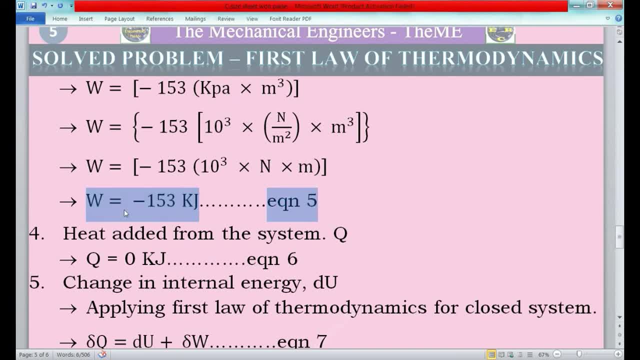 w is equal to minus 153 kilojoule. w is equal to minus 153 kilojoule. consider this one as equation 5. consider this one as equation 5. consider this one as equation 5. so so so the work done, the compression work during. 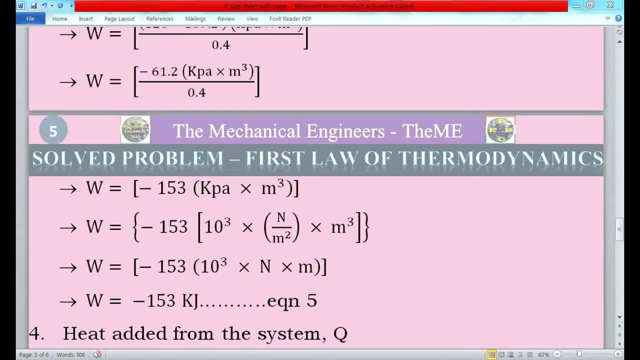 the work done. the compression work during the work done. the compression work during adiabatic process is adiabatic process is adiabatic process is minus 153 kilojoule. next we will find the minus 153 kilojoule. next we will find the. 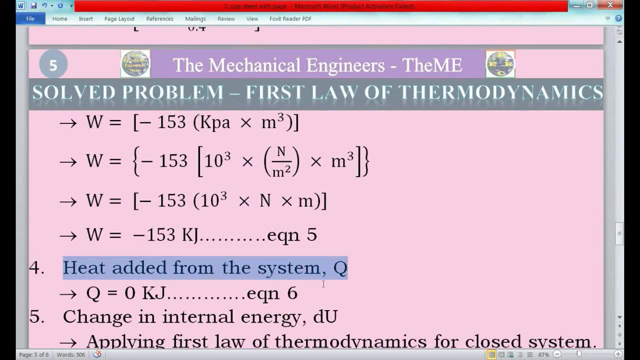 minus 153 kilojoule. next, we will find the value of heat added from the system. value of heat added from the system. value of heat added from the system, which is q- we know that. the compression which is q. we know that the compression which is q. we know that the compression of gas is carried out during adiabatic. 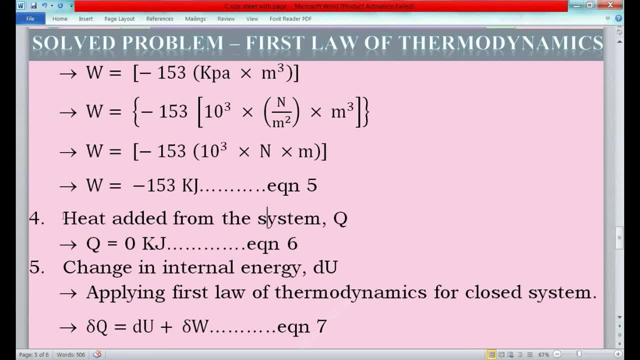 of gas is carried out during adiabatic of gas is carried out during adiabatic process process, process in adiabatic process. there will be no in adiabatic process. there will be no in adiabatic process. there will be no heat addition or heat rejection. 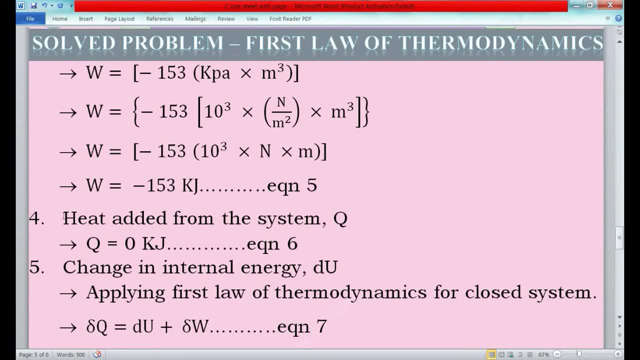 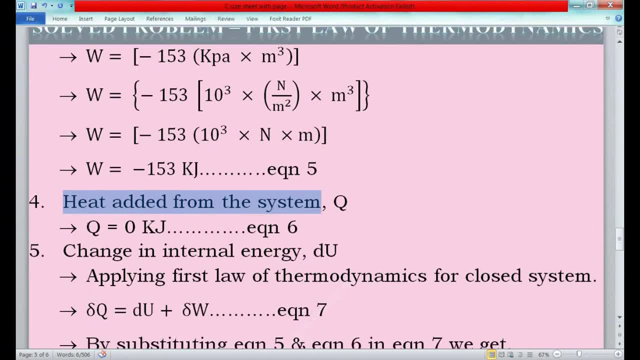 and also there will be no heat rejected. and also there will be no heat rejected from the system. therefore, the heat added from the system, therefore, the heat added from the system, therefore, the heat added from the system will be q is equal to 0 from the system will be q is equal to 0. 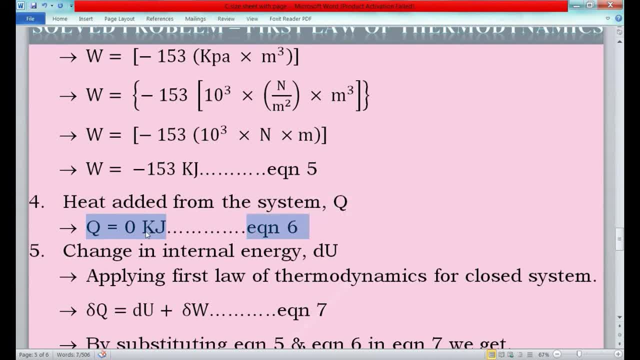 from the system will be: q is equal to 0 kilojoule, kilojoule, kilojoule. and consider this one as equation 6. and consider this one as equation 6 and consider this one as equation 6. now we will find the value of change in. 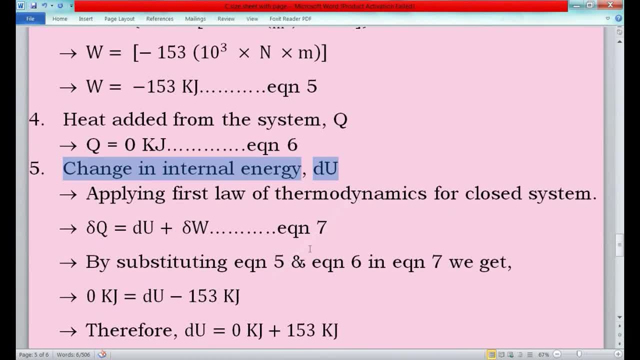 now we will find the value of change. in now we will find the value of change in internal energy, which is du internal energy, which is du internal energy, which is du for finding the value of change. in for finding the value of change in, for finding the value of change in internal energy, we are going to use the 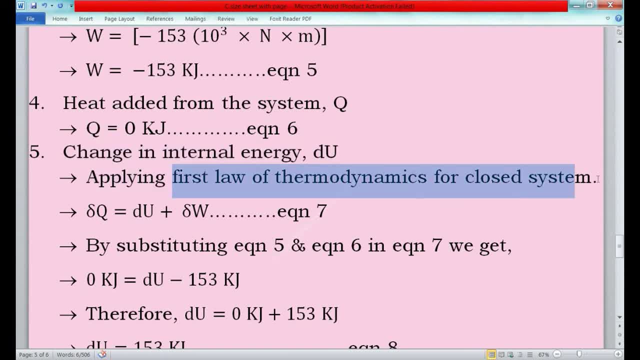 internal energy. we are going to use the internal energy. we are going to use the formula of first law of thermodynamics, formula of first law of thermodynamics, formula of first law of thermodynamics for closed system, and the formula is for closed system and the formula is: 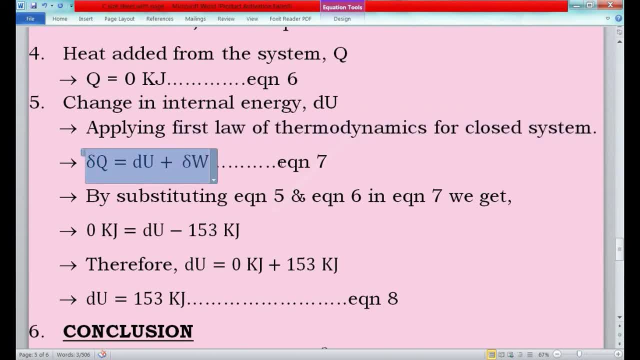 for closed system and the formula is: dou q is equal to du plus dou q is equal to du plus dou q is equal to du plus dou w. consider this one as equation 7 dou w. consider this one as equation 7 dou w. consider this one as equation 7. now substitute equation 5 and equation. 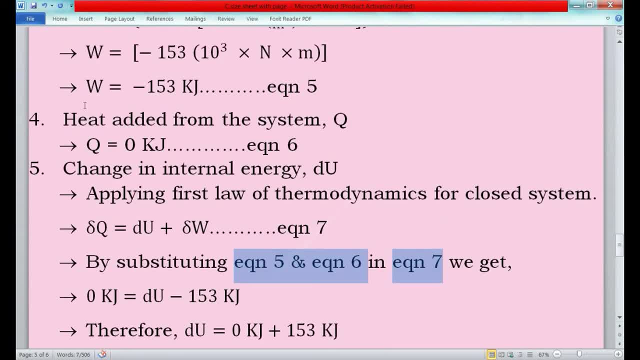 now substitute. equation 5 and equation now substitute: equation 5 and equation 6 in equation 7. 6 in equation 7, 6 in equation 7. what is equation 5? equation 5 is work. what is equation 5? equation 5 is work. 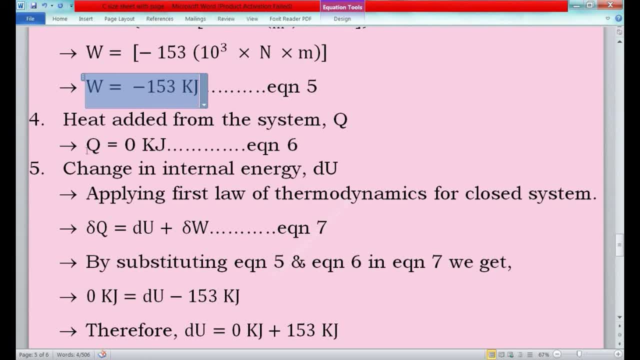 what is equation 5? equation 5 is work done which is minus 153 kilojoule, done which is minus 153 kilojoule. done which is minus 153 kilojoule. and equation 6 is heat added from the. and equation 6 is heat added from the. 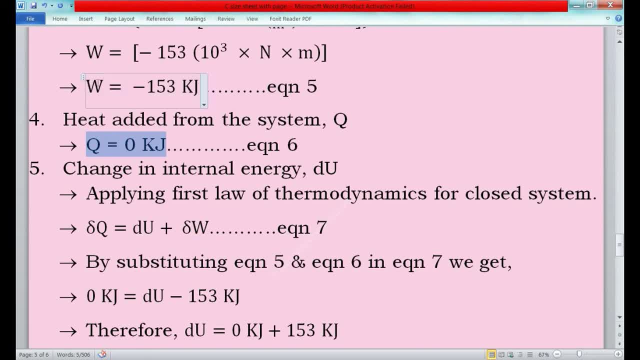 and equation 6 is heat added from the system which is q equal to 0 kilojoule system which is q equal to 0 kilojoule system which is q equal to 0 kilojoule. so substitute these two values in this. 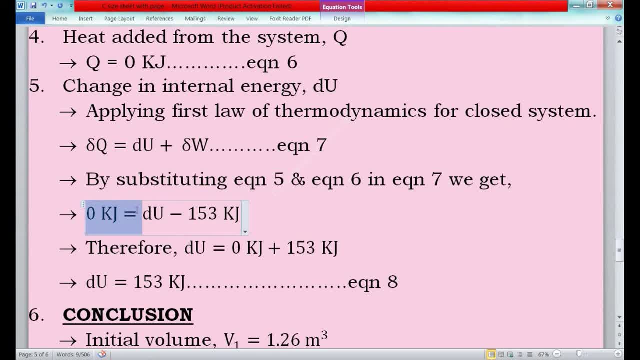 so substitute these two values in this. so substitute these two values in this formula formula. formula: we get 0 kilojoule is equal to du minus. we get 0 kilojoule is equal to du minus. we get 0 kilojoule is equal to du minus 153 kilojoule. 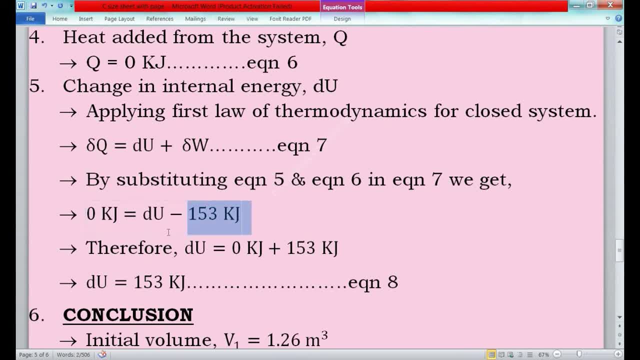 153 kilojoule. 153 kilojoule now. bring this 153 kilojoule to the lhs. now bring this 153 kilojoule to the lhs. now bring this 153 kilojoule to the lhs. we get du is equal to 0 kilojoule plus. we get du is equal to 0 kilojoule. plus we get du is equal to 0 kilojoule plus 153 kilojoule, so 0 kilojoule plus 153, 153 kilojoule, so 0 kilojoule plus 153. 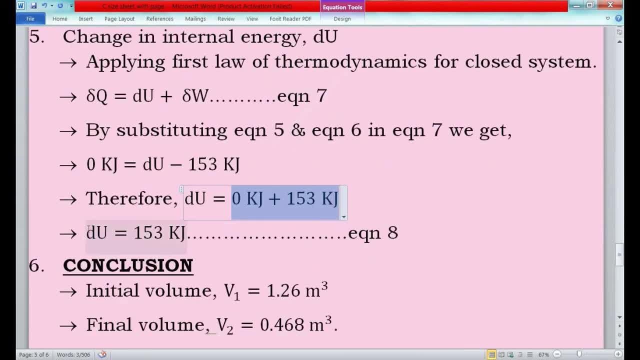 153 kilojoule. so 0 kilojoule plus 153 kilojoule is 153 kilojoule. therefore, the kilojoule is 153 kilojoule. therefore, the kilojoule is 153 kilojoule. therefore, the change in internal energy. 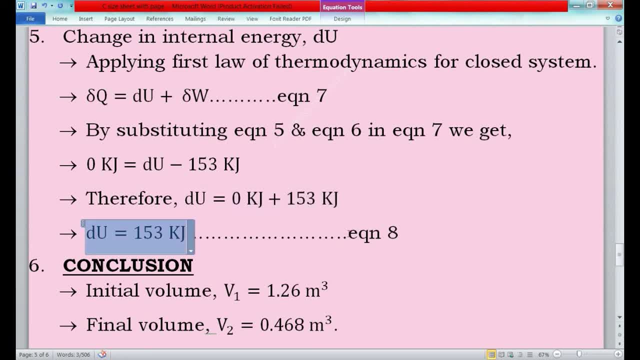 change in internal energy. change in internal energy: du is 153 kilojoule. consider this one as du is 153 kilojoule. consider this one as du is 153 kilojoule. consider this one as equation 8, equation 8, equation 8. so i have founded all the values. so it's. 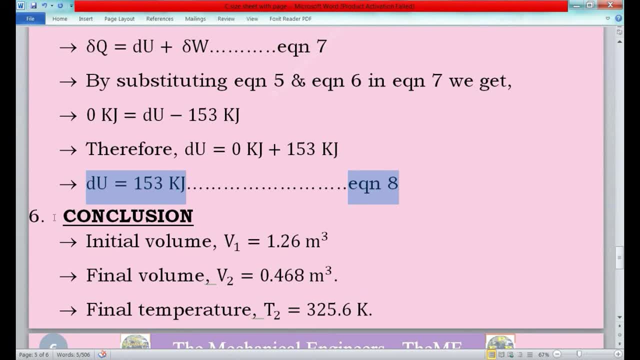 so i have founded all the values. so it's so i have founded all the values, so it's time to list out the solutions, time to list out the solutions. time to list out the solutions, which mean the conclusions, which mean the conclusions which mean the conclusions, is equal to 0.468 meter cube. 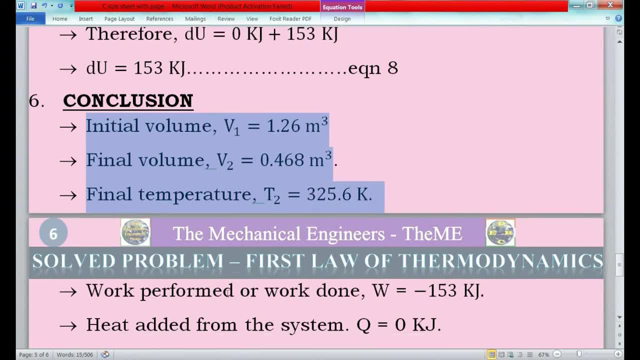 is equal to 0.468 meter cube is equal to 0.468 meter cube and the final temperature value is t2 is. and the final temperature value is t2 is, and the final temperature value is t2 is equal to 325.6 kelvin. 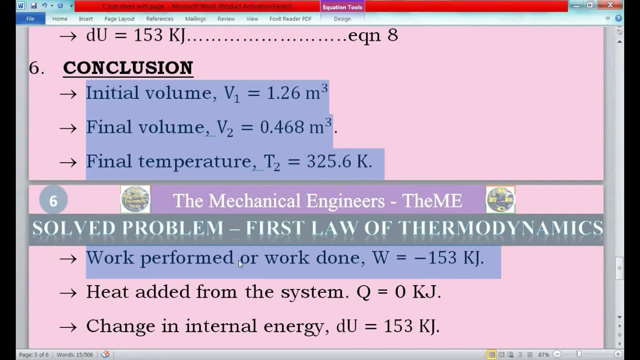 equal to 325.6 kelvin. equal to 325.6 kelvin and the work performed or work done is w, and the work performed or work done is w, and the work performed or work done is w is equal to minus 153 kilojoule. 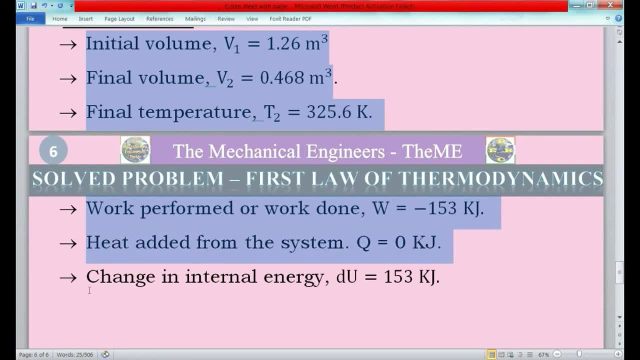 is equal to minus 153 kilojoule is equal to minus 153 kilojoule. the heat added from the system is q. is the heat added from the system is q. is the heat added from the system is q is equal to zero kilojoule. 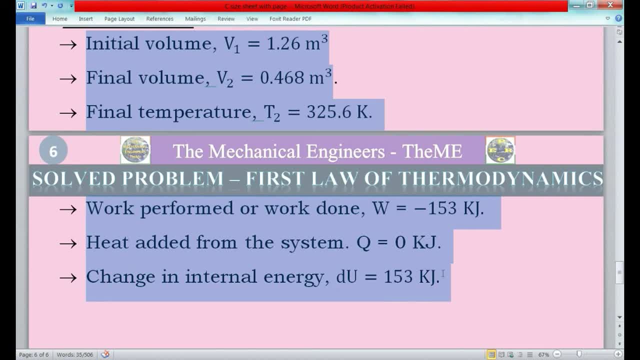 equal to zero kilojoule. equal to zero kilojoule. and the change in internal, the change in and the change in internal, the change in internal energy: is du is equal to 153. internal energy: is du is equal to 153. internal energy: is du is equal to 153 kilojoule. 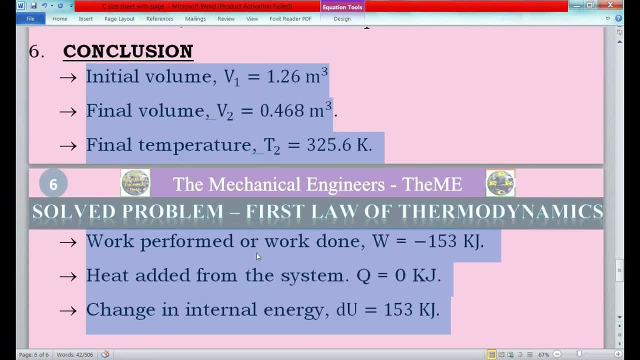 kilojoule, kilojoule. so these are the list list of solutions. so these are the list list of solutions. so these are the list list of solutions for this question, for this question, for this question. okay, so this brings an completion of. okay, so this brings an completion of.